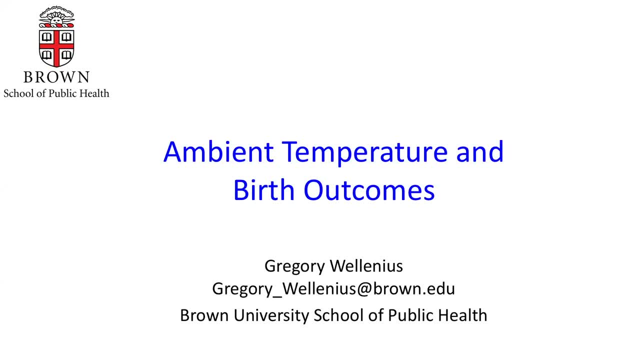 for 70 minutes and is being recorded for a call and webinar archive. With that, I'll turn things over to you, Ted. Thank you very much, Hannah, and let me extend my welcome. Welcome to all who have joined us as well today, As Hannah mentioned. 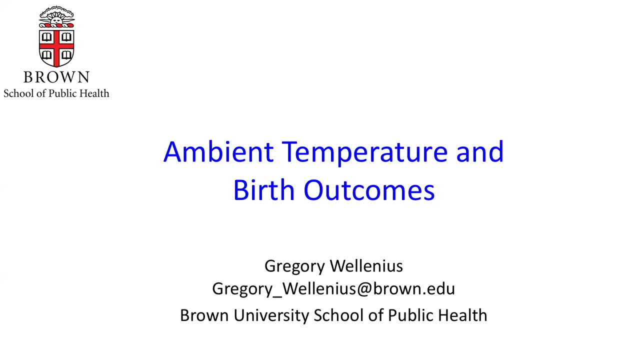 this is the first of four webinars on climate change and health impacts, and the other three are going to be touching on air pollution, extreme weather events and infectious diseases and their relationship to climate change, so stay tuned for those. Today we're talking about climate change and heat and health impacts. 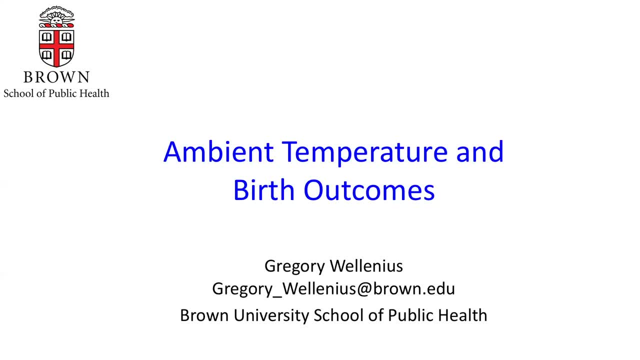 and we have with us three speakers, and what I'm going to do is introduce each of the three at the outset and then we'll go right into their presentations. The first speaker is Dr Greg Wallenius, Associate Professor of Epidemiology at the. 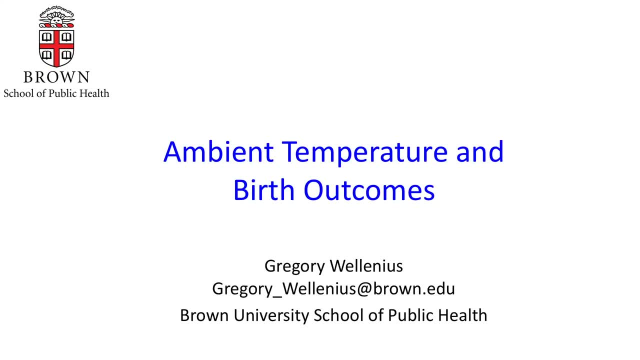 Brown University School of Public Health and Director of Brown's Center for Environmental Health and Technology, Dr Wallenius will present a brief summary of the associations between ambient temperatures and birth outcomes. Dr Wallenius recently served as co-author of the Fourth 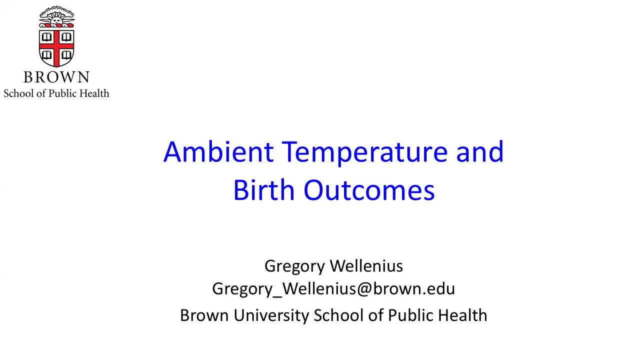 National Climate Assessment recently published by the US Global Change Research Program and is a member of the Rhode Island Climate Change Coordinating Council Advisory Board. Our second speaker, Dr Rish Vayanathan. excuse me for butchering that. 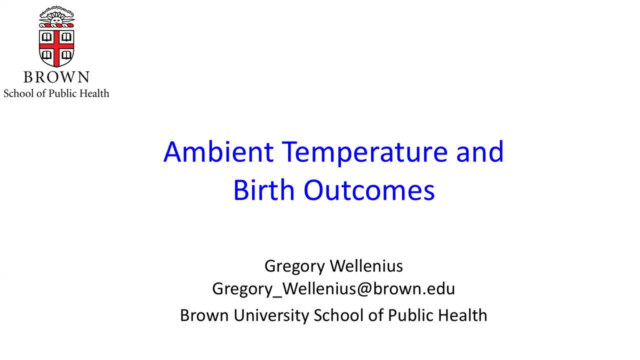 Dr Vayananathan is a health scientist with the Centers for Disease Control and Prevention. He has been working with the National Center for Environmental Health at CDC for over 14 years. His training and work experience include environmental engineering, epidemiology, data science and geographic information systems. 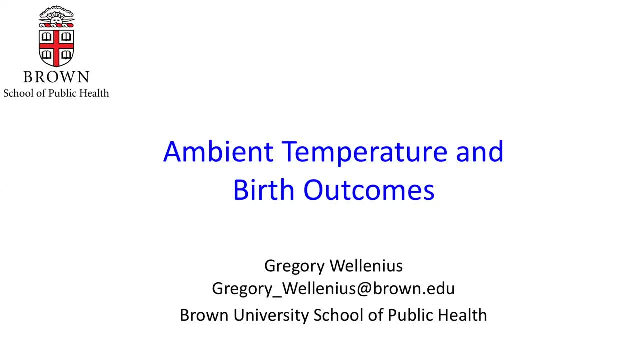 He has established collaborations with various academic institutions and other federal agencies on efforts to identify and characterize populations vulnerable to adverse health impacts from environmental stressors. He will discuss his publication Assessment of Extreme Heat and Hospitalizations to inform early warning systems. And our third speaker is Dr Eunice Lowe, a research associate at the University of Michigan. 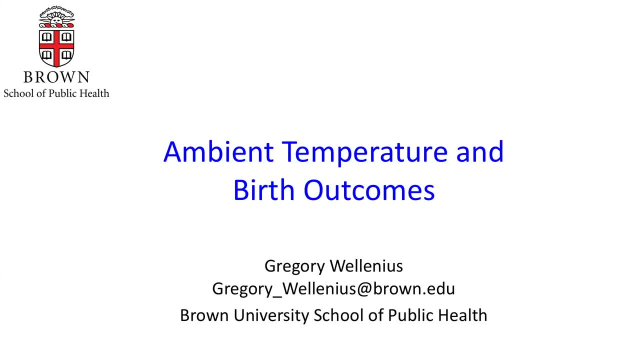 She is a professor at the University of Bristol and a member of the Cabot Institute for the Environment. Her expertise includes future climate change and changes in extreme weather events, with a particular focus on heat waves and their impacts on human health. Eunice received her PhD in Atmosphere, Oceans and Climate from the University of Reading. 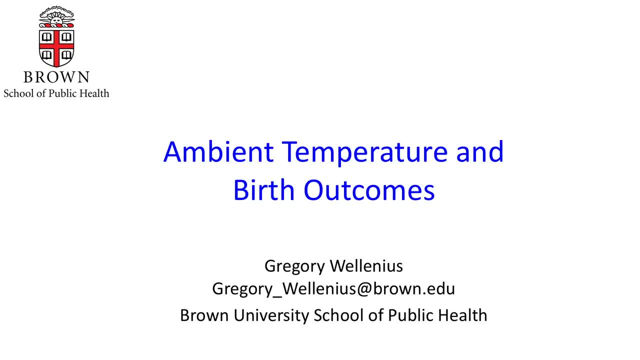 Adding to her background in climate science, she has a track record in science communication. Dr Lowe is a professor at the University of Michigan. Dr Lowe will present her research looking at differences in city-level heat-related mortality between the current 3-degree sonograde trajectory compared with a 2- and a 1.5-degree warming scenario. 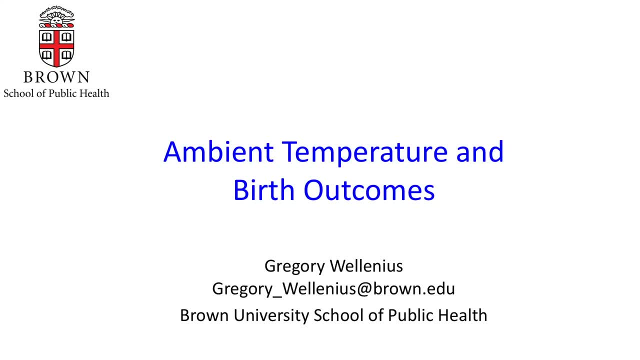 So with that as an introduction, Dr Velenius, please go ahead. Okay, thank you. Thanks, Ted and Hannah, for your warm welcome and for the invitation to speak today, and thanks to all of you that have joined the webinar. 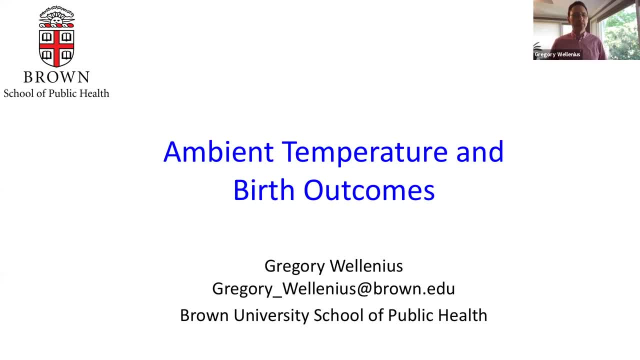 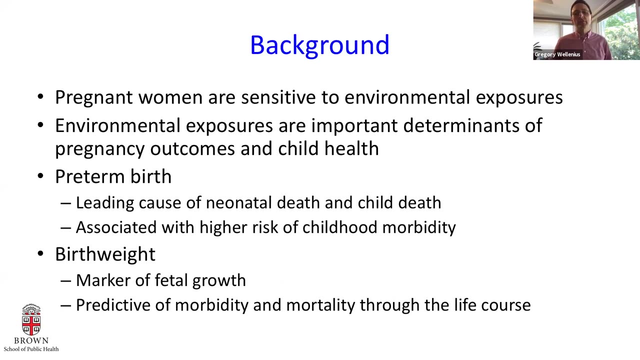 So my title is probably a little bit more expansive than I can cover in 15 minutes. There's a large, more emerging literature quickly getting large on ambient temperature and birth outcomes, And I'm only going to be able to talk about a small part of that, as relates to our recent and ongoing work in this area. 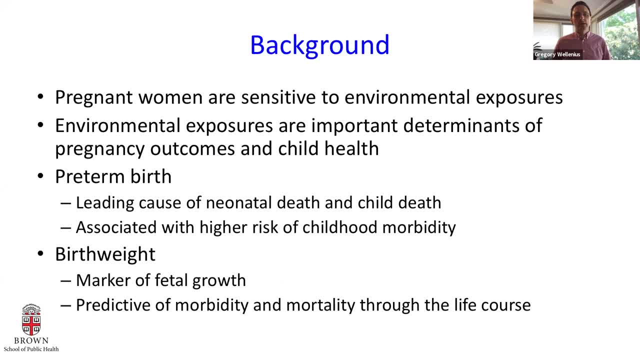 So there's a large literature showing that pregnant women are sensitive to, particularly sensitive to, environmental exposures- This is true of chemical exposures, air pollution, exposures in the medical environment or clinical environment- And that it's just becoming clear that this is a sensitive window of susceptibility for environmental impacts. 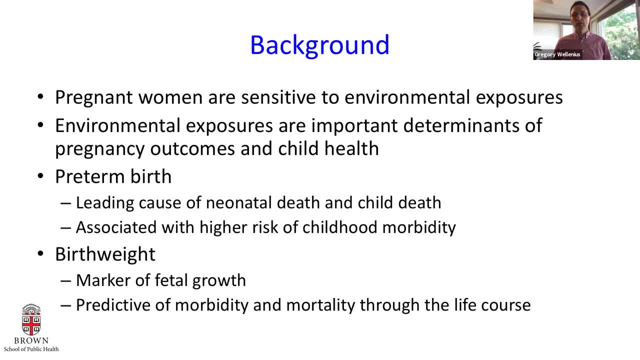 and that those impacts are not just on the mom during the pregnancy, but then on the pregnancy outcomes, and short- and long-term health of the child is potentially affected. Two specific birth outcomes that I want to talk about today are the risk of preterm birth and impacts on fetal growth. 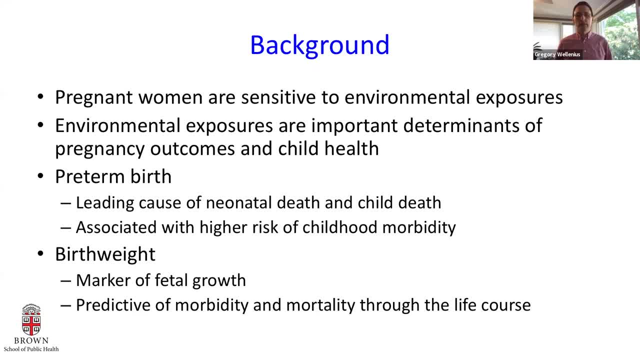 For preterm birth. it's one of the leading causes of neonatal death and child death in particularly children under five years old. It's the leading cause And it's associated, again, not just with sort of an acute risk around the peripartum time, but also. 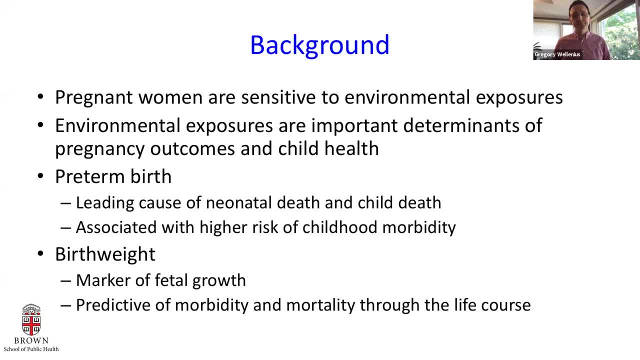 with long-term impacts on childhood morbidity. Birth weight has a very long history as a marker of fetal health and an important birth outcome that's tracked clinically. It's obviously a marker of fetal growth and it's predictive of morbidity and mortality throughout the life course. And of course we've heard a lot about life course epidemiology in recent years and sort of. 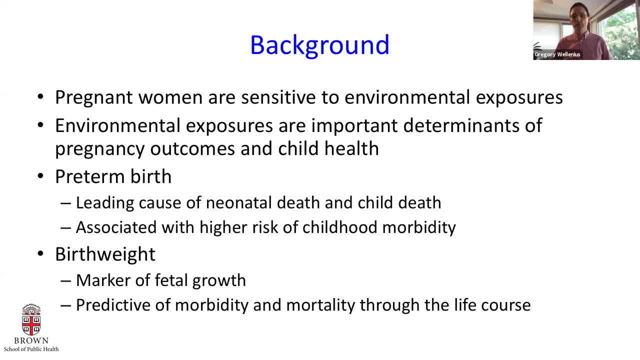 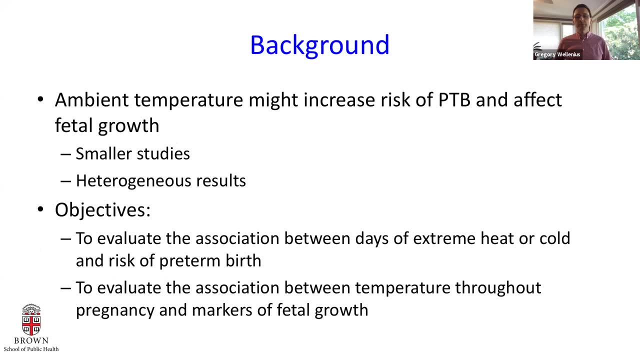 the thought that you have these susceptible windows of exposure early and late in life. That then determines your disease risk or your health status for potentially setting you on trajectories that last a lifetime. So ambient temperature might increase the risk of preterm birth and also impact fetal growth. There's been a number of studies on this question already, and 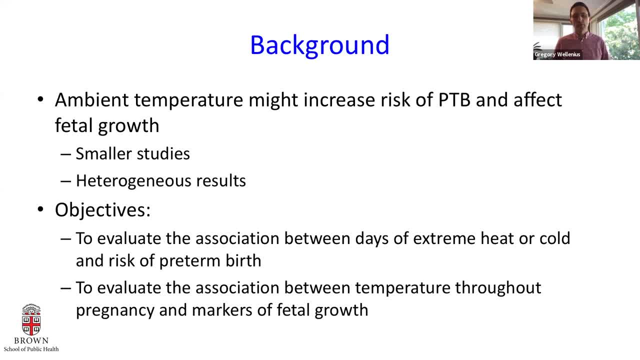 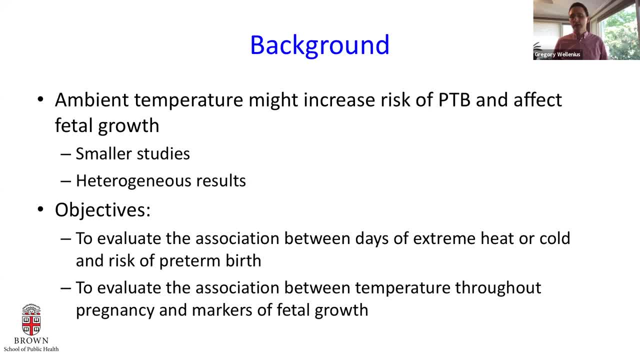 Fetal growth associated with temperature. but the results have been quite variable. So there seems to be variability depending on where you do the study and maybe different methods and approaches to looking at that question. So our objectives were to evaluate the association between days of extreme heat or cold and risk of preterm birth. So that's the sort of short term in just the two to four days right before. 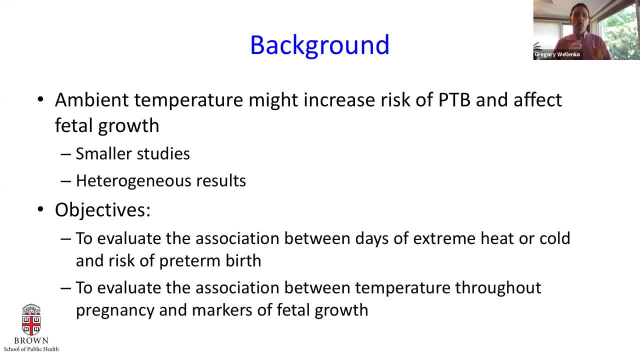 So two to four days of extreme heat or cold. does that lead to triggering of preterm birth? And, separately from that, to evaluate the association between temperature throughout pregnancy and markers of fetal growth? So now we're talking about a slightly different time scale, talking about temperature averaged over the whole pregnancy or in specific trimesters. 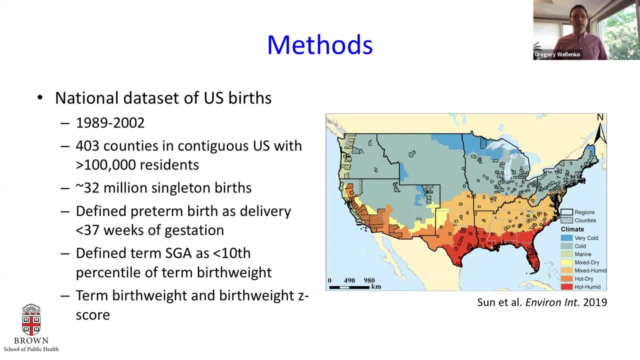 So we performed both of these studies within a national data set of US births obtained from the CDC. These were births from 1989 to 2002 in 403 counties in the contiguous US, and these are counties that are deemed large enough by the CDC that they could release this information at. 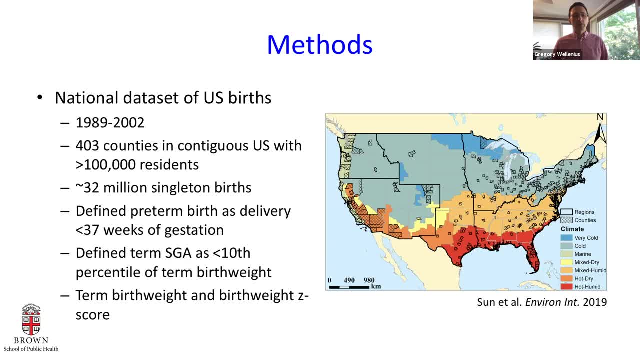 the county level without risk of being able to re-identify individuals. And during this time period, across these 400 counties there's about 32 million singleton births. You can see in the figure on the right you can see the output and the monoculture. on the left the proportion of births, And for this we could 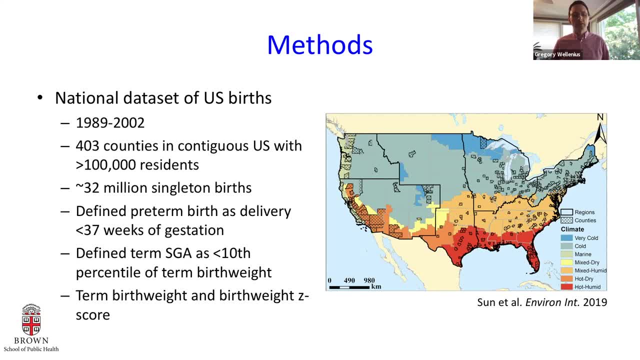 outlines of the counties involved, and then the bigger outlines are the outlines of the national climate assessment region, so that we can look at regional effects as well as national effects. And then you can also see that we defined different climate types according to the colors scheme you see on the axis there. We defined preterm birth as the standard definition. 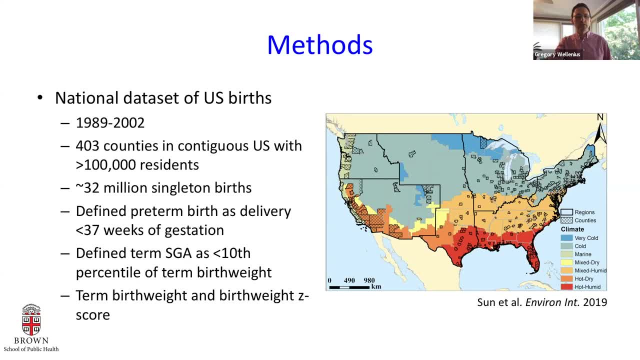 of delivery prior to 37 weeks of gestation And then for looking at patterns of fetal growth. we define term small for gestational age as those babies in the bottom 10th percentile for term birth weight. So this is amongst term births only And then term birth weight. 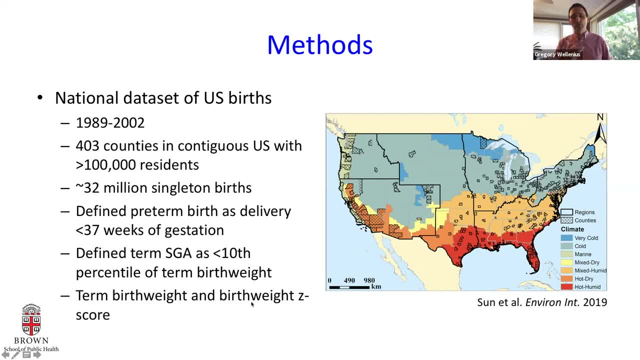 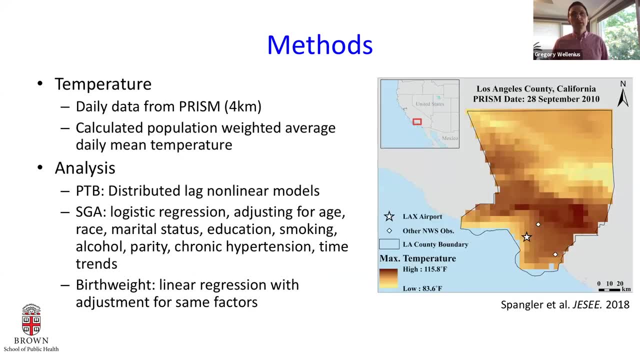 just as a continuous variable, but also the birth weight Z score, which adjusts or accounts for gestational age at the time of birth, Again amongst term births. So we needed there's a number of ways that you can think about what temperature people are exposed to across the country. We chose to use an. 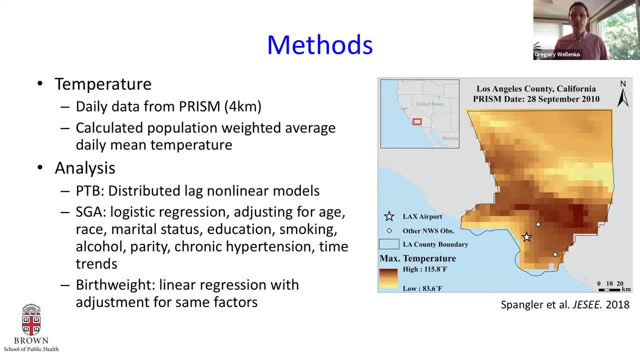 approach that we've described recently. This is the PRISM dataset produced by Oregon State University, and it's at a four kilometer resolution. Here you can see one day in one particular location in the Los Angeles area. It's a county on the west coast, obviously, And so you can see that even within a county. 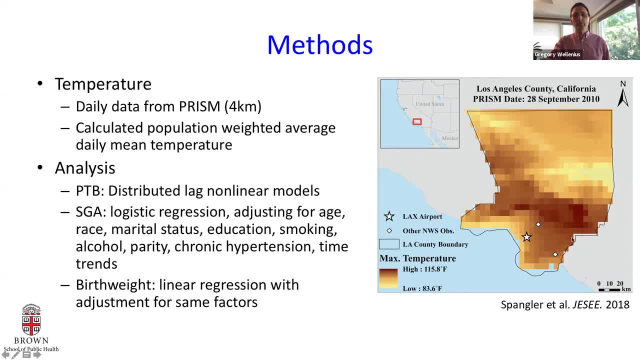 each grid cell here is four kilometers. by four kilometers There's quite a bit of variation in temperature even within the county, And what we did is calculated for each county: the population weighted average, daily mean max and min temperature For today. I'm going 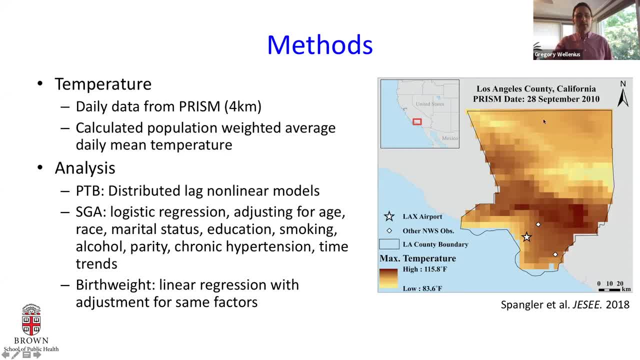 to focus only on our use of mean daily temperature averaged at the county level, And then, in terms of analyses, I'm happy to go into more details if there's questions. It's well described in the paper as well. But for the looking at the risk of preterm, 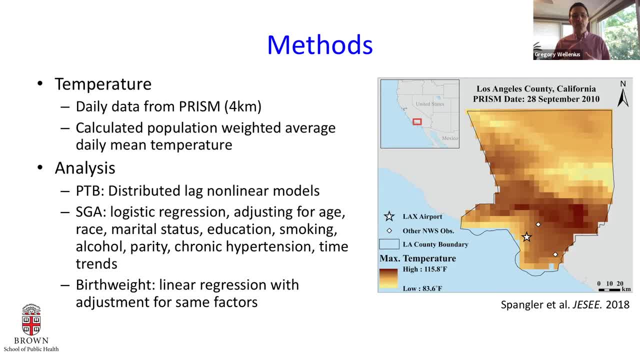 birth in response to a couple of days of extreme weather, we use distributed lag nonlinear models. These are now a well established framework that allows you to look at multiple days of exposure And with a flexible nonlinear framework. So that's described in detail there in the paper. 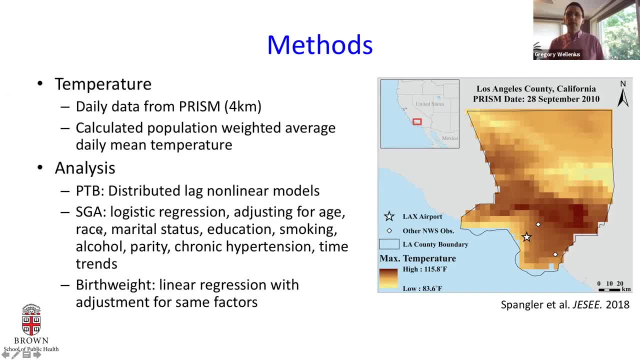 obviously, Then for looking at the risk of small for gestational age. Now, remember the time period we're looking at. there is the whole pregnancy, or trimester, specific averages. So there we just use logistic regression looking for each birth. Was it small for gestational age or? 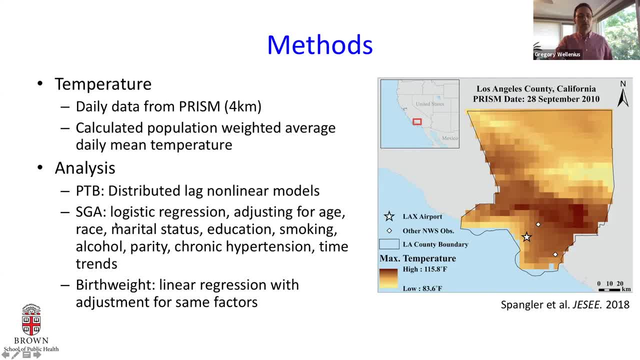 not Yes or no, And then all models were adjusted for age, race, marriage, gender and age. And then we looked at the risk of small for gestational age. Now remember the time period we're looking at. there is the whole pregnancy or trimester, specific averages. So there we. 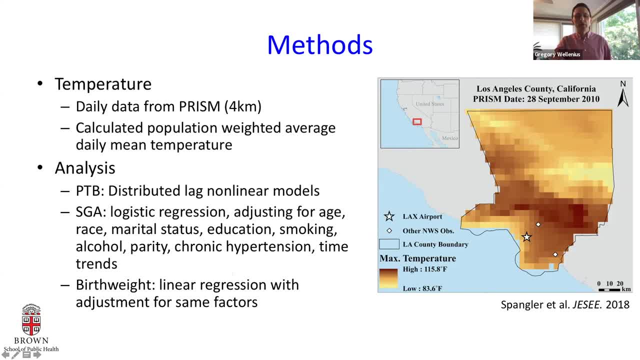 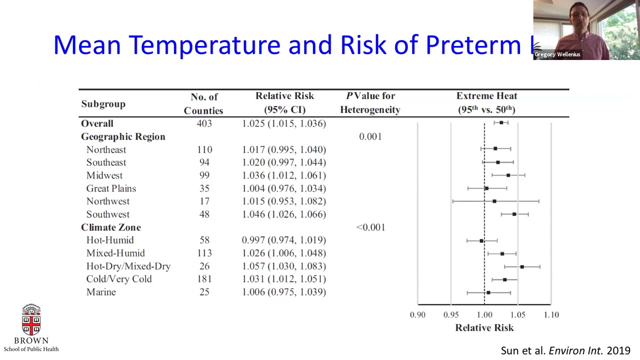 just use logistic regression looking for each birth. Was it small for gestational age or dlae? That's a pretty straightforward argument. We did look at both preterm birth and gestational age. So, like I said before, But without helped with all of that, we can't tester this. After all, we're looking at 15 extra hours. 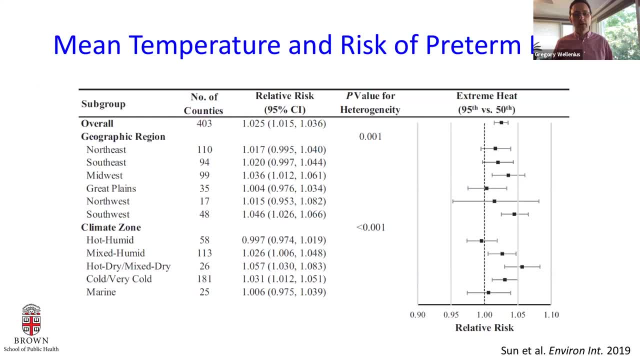 risk of preterm birth. This is about a two and a half or three percent increase in the risk of preterm birth on days of extreme heat. This is the 95th percentile or above, compared to the 50th percentile of temperature for that county And we looked at. this. effect varies across geographic. 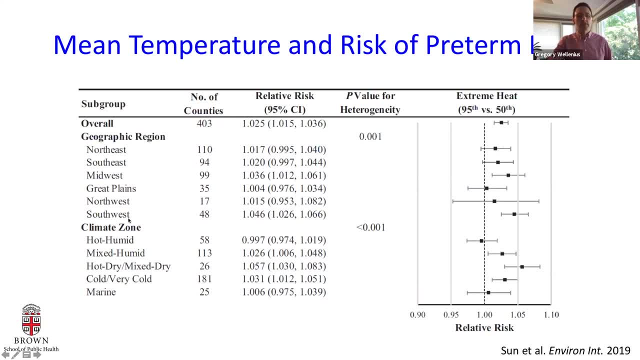 regions of the country. So these are the national climate assessment regions that, for the contiguous US, that we used And you can see that the strongest associations are seen in the southwest, in the midwest and in climate zones that are considered to be hot, dry or mixed dry. 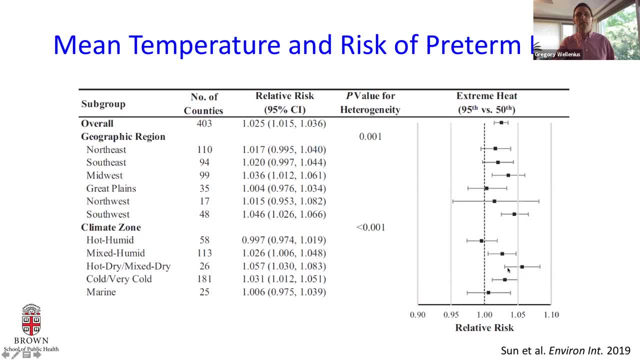 So there's some regional variability, which is interesting to think of how prior studies that have been done in smaller locations or across smaller regions have been done, And so this is interesting to think of how prior studies that have been done in smaller locations or across smaller 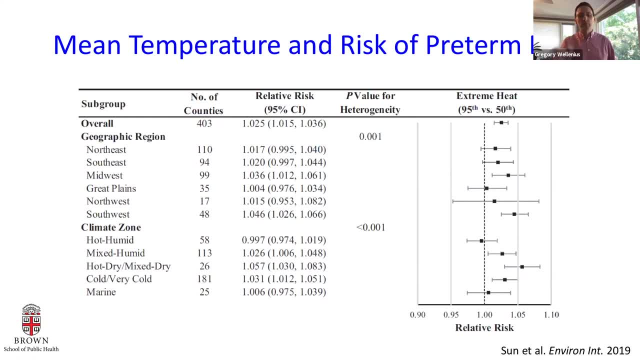 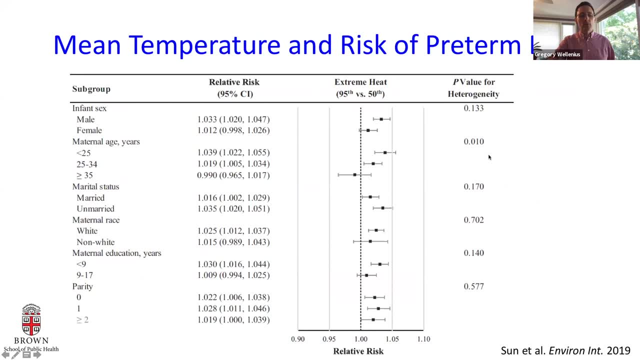 spatial extents might be in part variable because of the differing effects by geography and typical weather. We also looked at whether there was effect modification by individual level characteristics, And so, as you can see here- and the one I want to point your attention to is that- 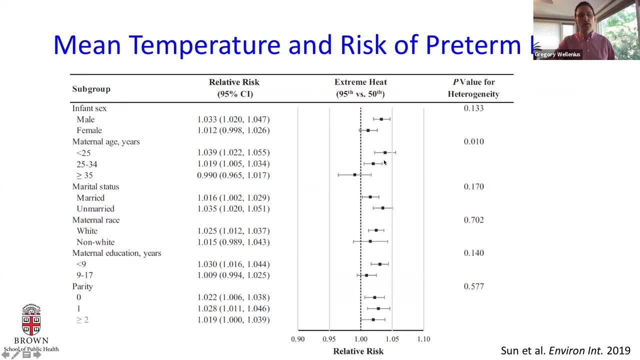 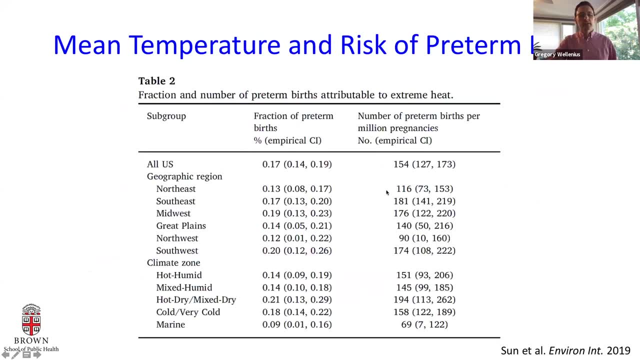 younger women seem to be at greater risk of preterm birth, And so this is a very interesting scripture based on a sample from 2013, where they kind of More national numbers forDid progress to that data, but the average represent stationary aircraft呔 on very hot days And, given this association, we can say: if this association we're 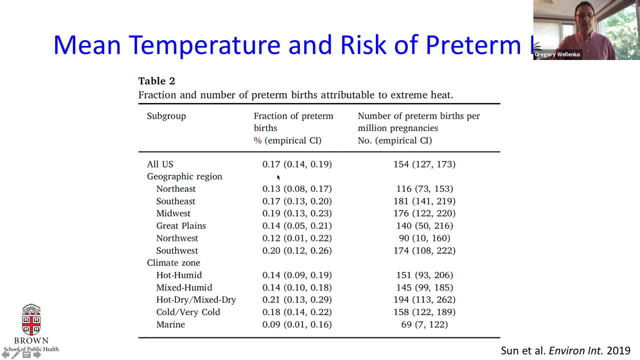 seeing between days of extreme heat and risk of preterm birth. if that is causal, the determination that we need to make based on the totality of evidence. but let's just symmetric: ング. gib is the fraction of preterm births due to extreme heat, and then here the number of preterm births. 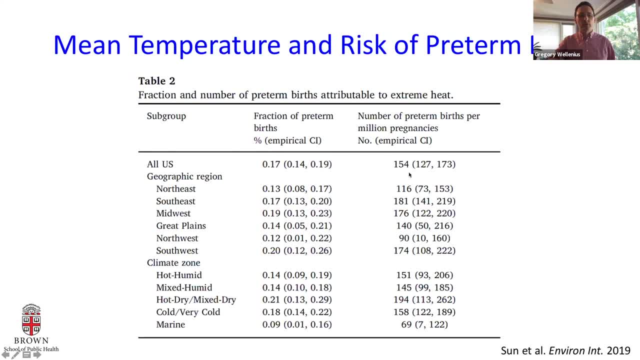 per million pregnancies for either all of the US in the top row or by region of the US or by climate zone, And so you can see that about 154 per million births there might be about 154 preterm births that are attributable to extreme heat, if these results indicate a causal effect of. 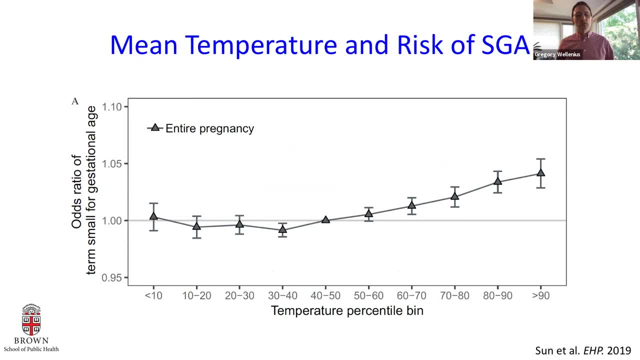 heat. So, moving on to fetal growth, remember we were looking at the temperature during, the average temperature across the pregnancy and the risk of small for gestational age. and again, we did this in percentiles because different counties have different typical weather and so we want to. 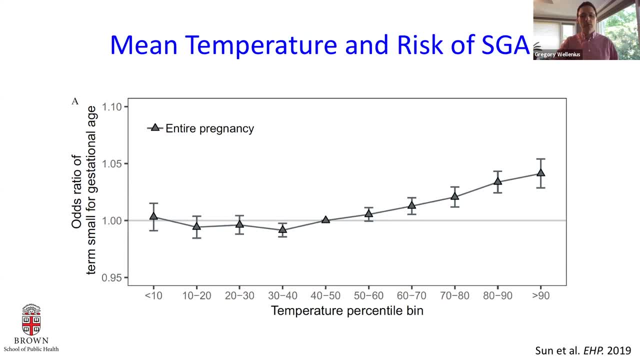 to do this relative to the weather that local people are accustomed to, and so when the pregnancies were in mean temperature- the pregnancies were sort of in the 90th top- you know, top 10th percentile of the pregnancies- there was a higher risk that was associated with a higher risk of small for. 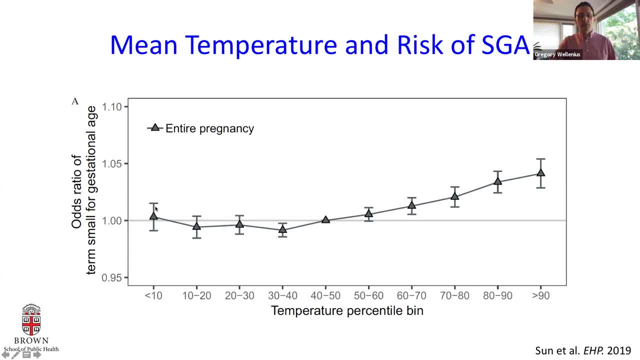 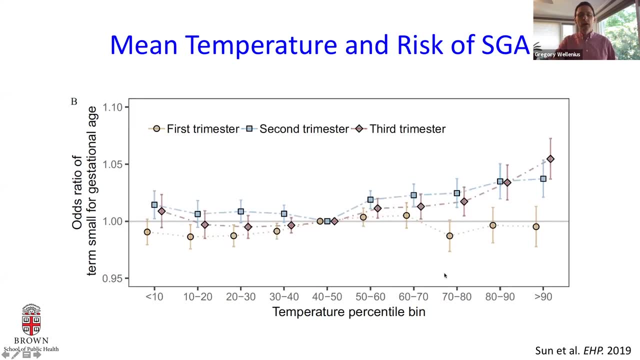 gestational age, with no similar effect on the cold end of the spectrum When we broke this in by trimester. so now we see that the association is present for mean temperature during across the third trimester and the second trimester, but not associated with mean temperatures. 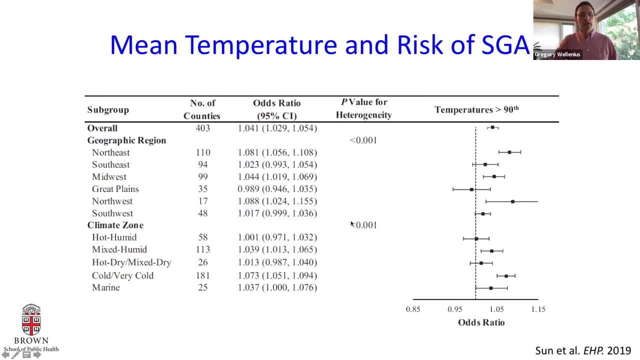 in the first trimester. Similarly, we looked at whether there were regional or climate zone differences in the associations we saw and here for the risk of SGA. we see stronger association in the northeast and the northwest and these are regions that are considered to have typically colder weather, so in the cold, very cold and marine environments. 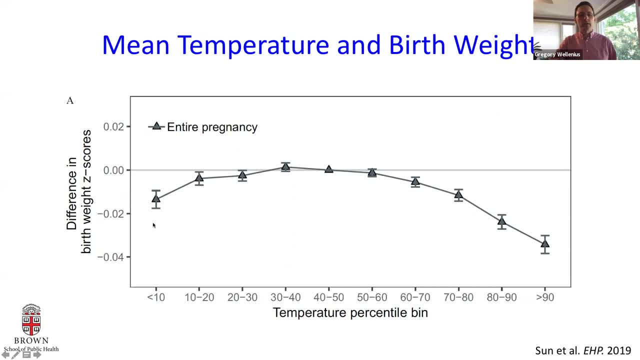 Hand in hand with that. we can look at birth weight. Here we have birth weight z score, so this is again standardized for gestational age of birth and here we see that hotter average temperatures during pregnancy are associated with a low, slightly lower, birth weight z score, as well as extreme cold temperatures are associated with. 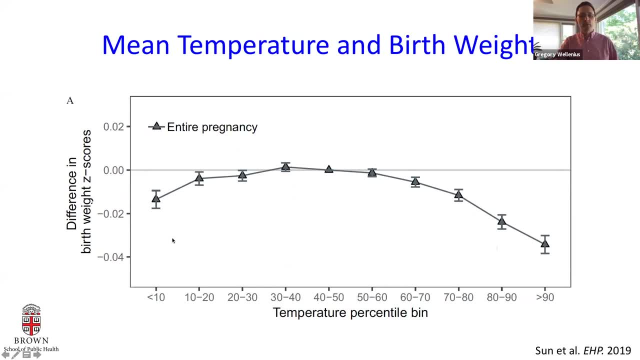 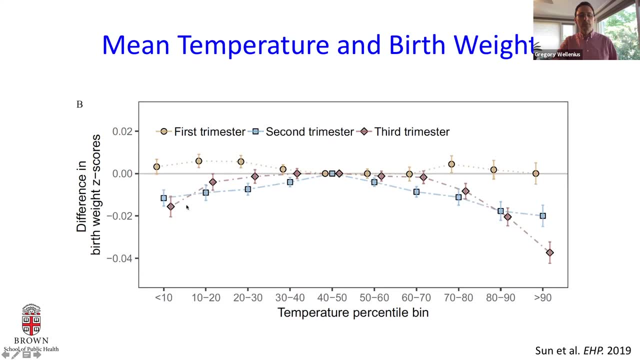 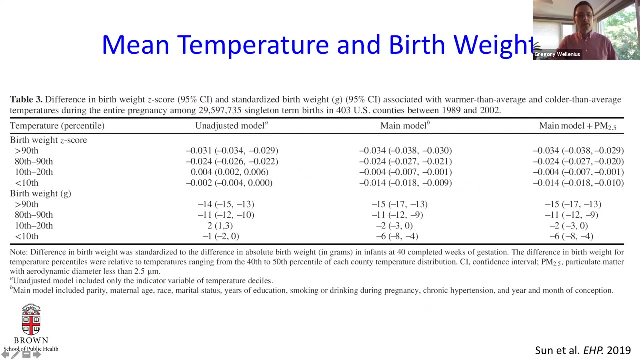 slightly lower birth weight z scores and again, as in for the risk of SGA, the association was most evident in with relationship to temperatures in the second trimester and third trimester and not associated with temperatures in the first trimester. Another way to to look at this is, of course, with sort of model coefficients for for specific 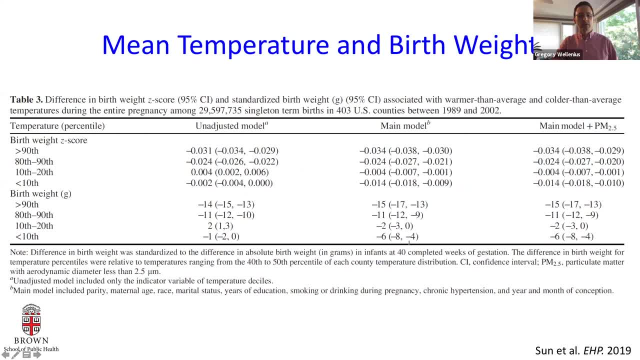 intervals, and so you can see particularly- I want to direct your attention to the bottom here, where we have birth weight in grams, just to give you an idea of the magnitude of the effect in a, in a number that we can relate to, and so we're talking about pregnancies in the warmest temper. 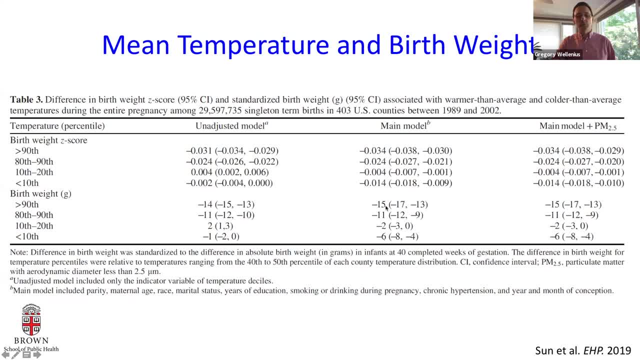 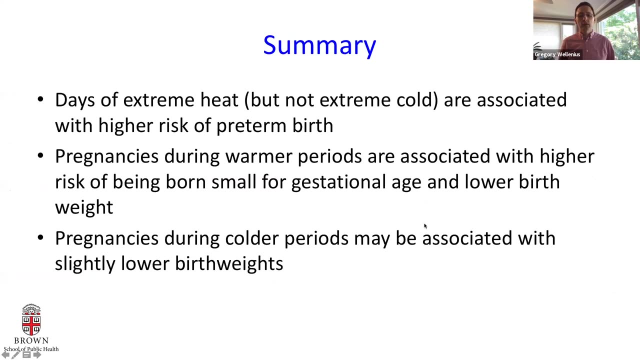 of the centile, being about 15 grams smaller compared to two pregnancies in the in the 40th, The 50th percentile of temperatures. so it's- I would describe that as a modest association. So, in summary, days of extreme heat but not extreme cold are associated with higher risk of preterm. birth. Pregnancies during warmer periods are associated with higher risk of being born small for gestational age and having lower birth weight, but pregnancies during colder periods the results warrant as consistent. they may be associated with very slightly lower birth weights, but not with increased risk of small for gestational age. As with all studies, we have strengths and limitations. 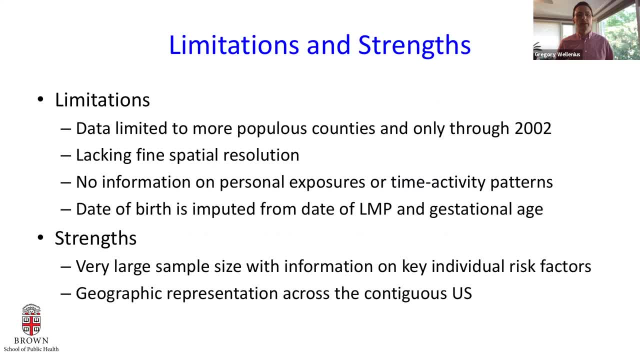 so our data were limited to those counties I showed you at the beginning but that were most populous, and the data are only available publicly at that geographic resolution through 2002.. So we're lacking a finer spatial resolution than county on the eastern half of the us. that's not. 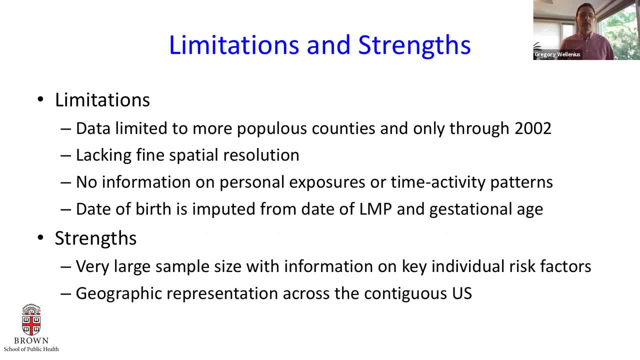 such a problem because counties tend to be small. in the western half of the us, counties tend to be quite a bit larger, and so there's a lot more of the information around this. I'm going to go ahead and just go from the way it is going down now. I'll just go from the way I can see them. I'm going to go. through the data. I'll just go through them bit by bit And I'll just go through each one of them, And I'll go through some of the data on the left side, in the upper left, and then I'll go through the data on the right side of the data. 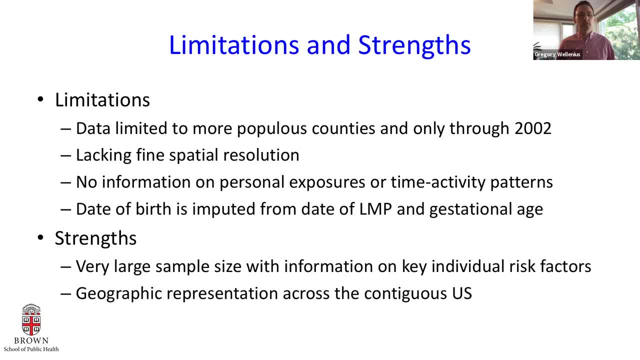 there's a missed opportunity there to do a finer spatial scale analysis. We have no information on what people were doing, whether they moved during the course of their pregnancy, or how much time they spend at home versus other locations, or, in fact, how much time they even spend outside the 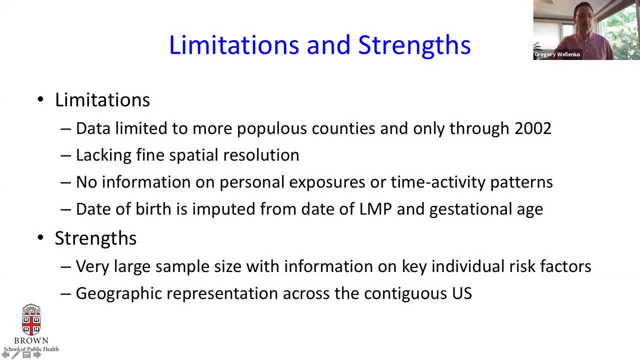 home, as is common in this type of population level study. And our date of birth? the date of birth isn't actually available in the data We imputed. it based on the date of the last menstrual period and the reported gestational age, So there's some potential for misclassification of. 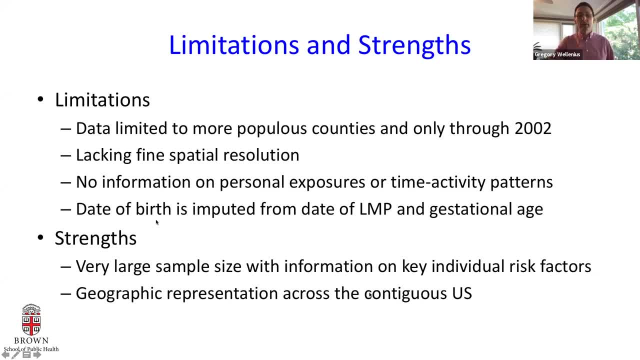 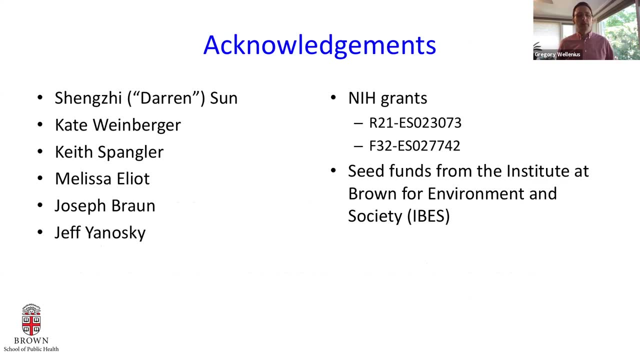 the date of birth. in both of these studies. On the other hand, we have a very large sample size with information on key individual risk factors and geographic representation across a very large area. Of course, this represents the culmination of work by a number of people, including 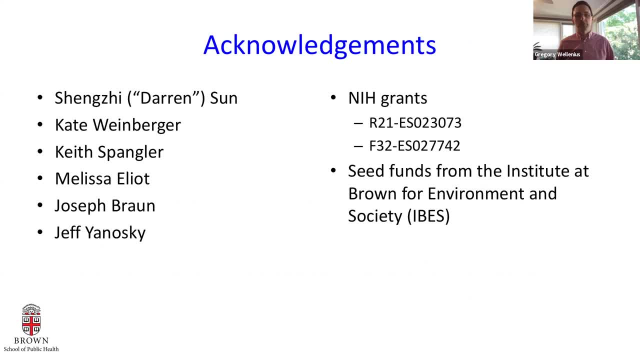 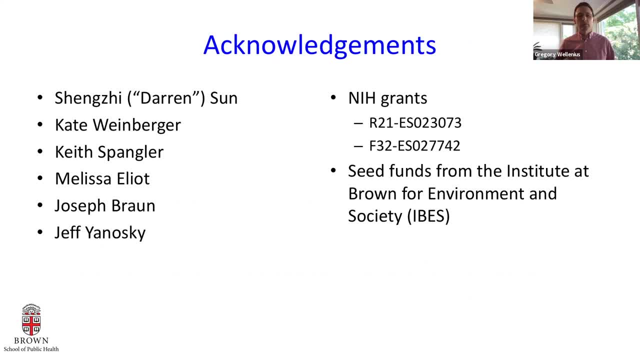 help and support from a number of other team members and, of course, funding from both government agencies and intramural support from the University. With that I'll stop. Thank you Great. thank you so much, Dr Vuolanos. 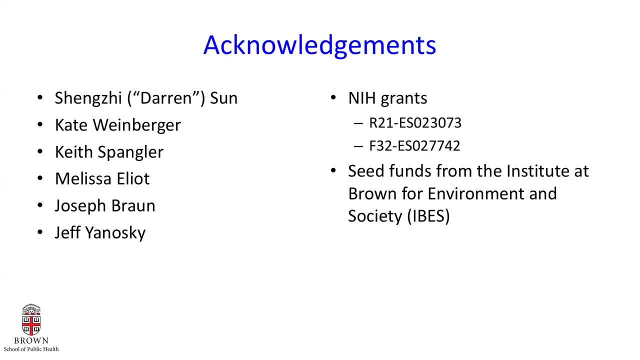 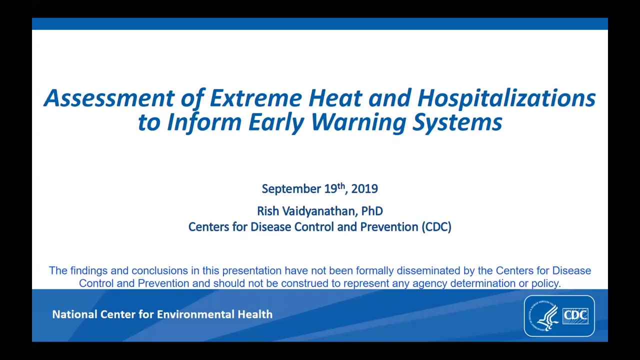 We're going to move on to Dr Гдеhanathan's presentation. just a moment here. He's going to pull up his slides And we'll be ready in just a moment. Dr Vedianathan, can you hear me? There we are. 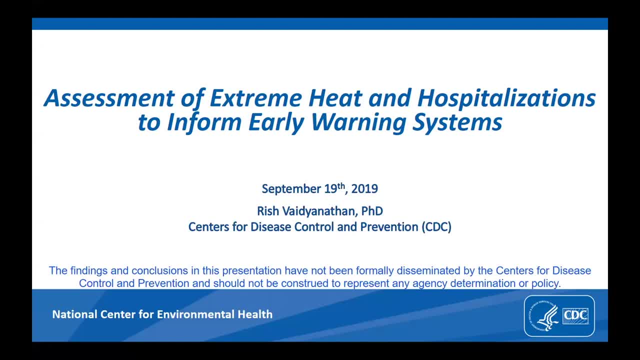 Yeah, I can hear you. Can you guys see my slide? Yes, Okay, All right, Thank you. Thank you, Hannah, and thanks for inviting me. Good afternoon and good morning wherever you are. So today I'll be presenting on our work assessing relationships between extreme heat and hospitalizations. 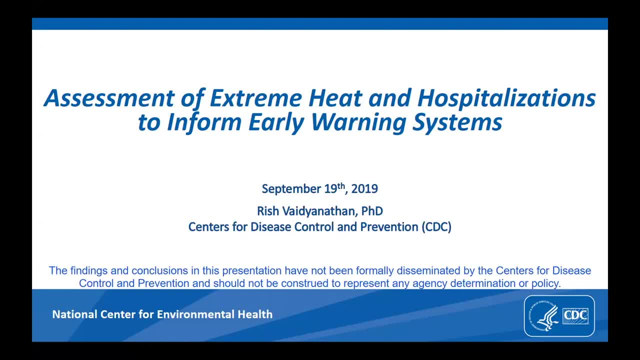 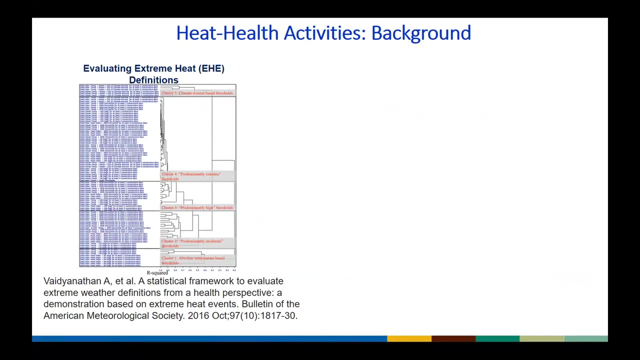 Basically the goal was to inform heat early warning systems, and the work presented here was recently published in the Proceedings of the National Academy of Sciences. And just to give a bit of background on our heat health work, we first started evaluating definitions of extreme heat events and basically to operationalize some long-term extreme heat. 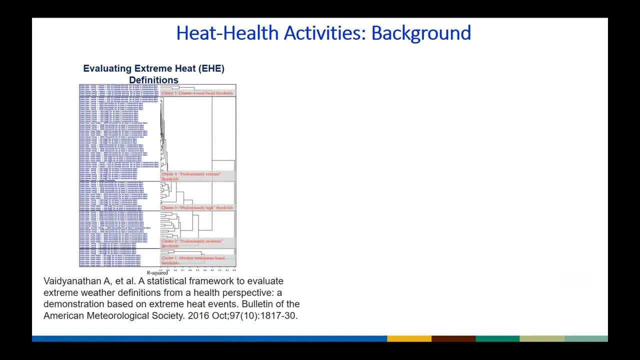 indicators as it relates to climate change, But then, based on our evaluation of the extreme heat events, we were able to determine what the extreme heat events were. So if we look at the Colorblind EHE definitions, one thing we noticed was how those definitions 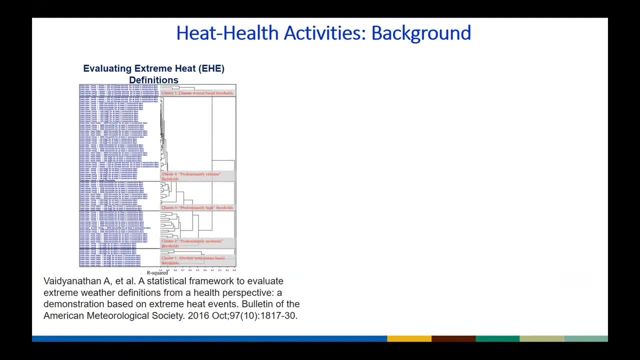 using extreme thresholds had poor associations with heat-related health outcomes. I mean, this is particularly evident in colder regions And this furthered our interest in understanding heat health relationships by various climate regions. And subsequently, when we had a meeting with the National Weather Service, you know, we 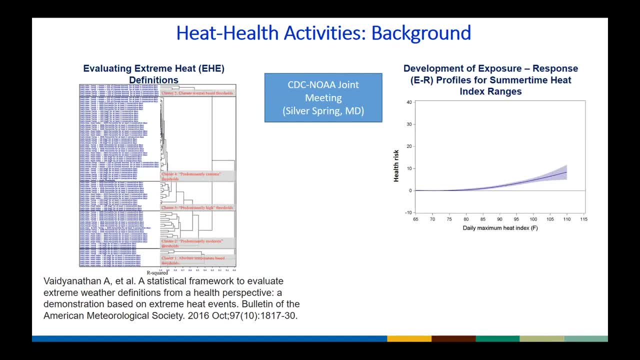 were told about how existing heat alert protocols work and how they use these things to monitor the climate thresholds and early warning systems for heat, and we also learned that alerts are mostly issued at very high temperatures, even in colder regions, and this was about five years ago. 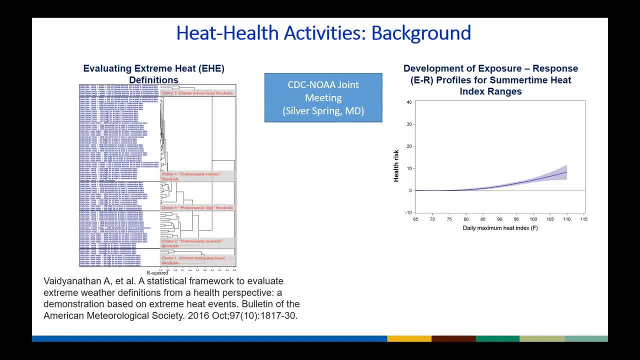 and further. in that meeting we also discussed about the possibility of how the health community can provide some evidence so that these epi data or information from epidemiologic analysis could inform existing heat alert products. so our interest also was to sort of look at health risks over a wide range of temperatures, basically to understand what's happening. 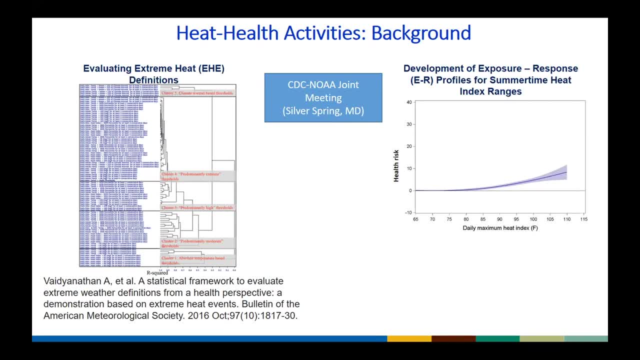 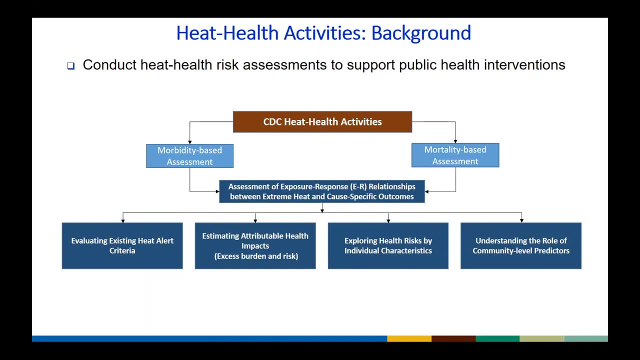 at moderately high heat index or temperature regimes, and this schematic reflects our thought process before, if you will, before, starting this project. I mean, in a sense, we wanted to generate health evidence based on both mortality and morbidity assessment and also to inform the following aspects. so first, obviously, we wanted to evaluate the existing heat alert. 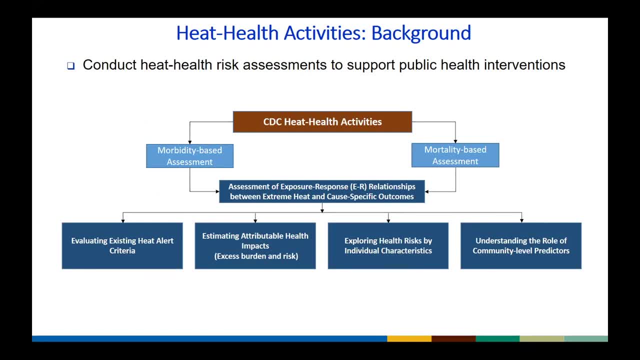 criteria. so I know I mean it's common knowledge that alerts are issued at extremely high temperatures. I mean it's been, you know, discussed fairly consistently now in the public health community. but comparing health risks and alert thresholds was necessary to highlight the disconnect that was prevalent mainly in the weather community and also we wanted to estimate attributable. 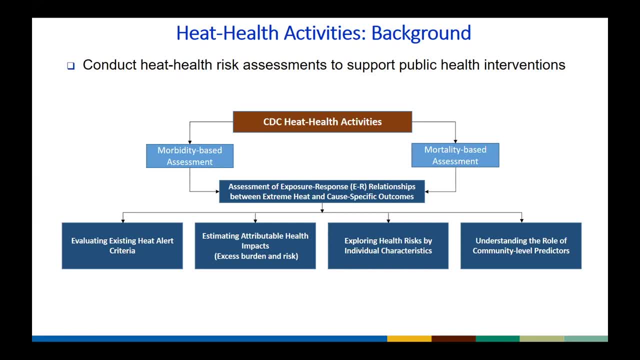 health impacts associated with heat, basically looking at measures of excess burden and risk rates and the risk factors within that area, and why that is a challenge, and sometimes what I learned from this project is that, in particular, we wanted to aim at addressing these types of health risks in a different way from the traditional ways of doing this. 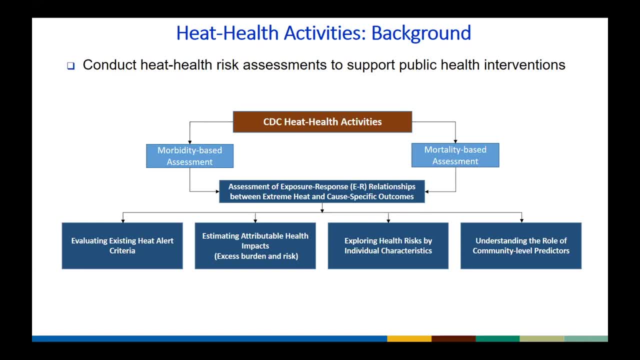 so sort of the communications, communication aspect of this becomes easier because, like you know, in the health community we're used to discussing things based on health risks, relative risks, all that. but then it's easier if you sort of present information by these burden estimates or the excess burden or excess number of debts or excess number of hospital admissions. 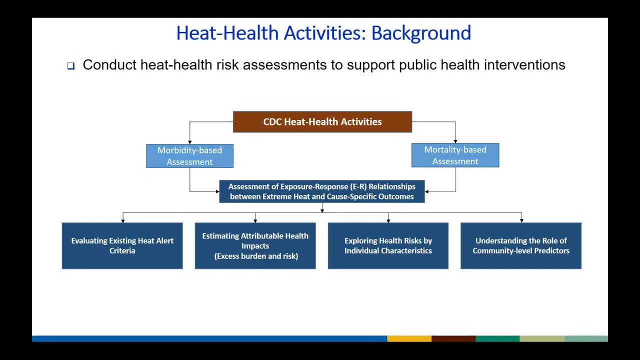 also understanding the role of community level predictors. So I guess these are all important things, but our goal was to sort of see how all this fits in with our overall scope of informing public health practice, And for today's presentation I'm just going to be focusing. 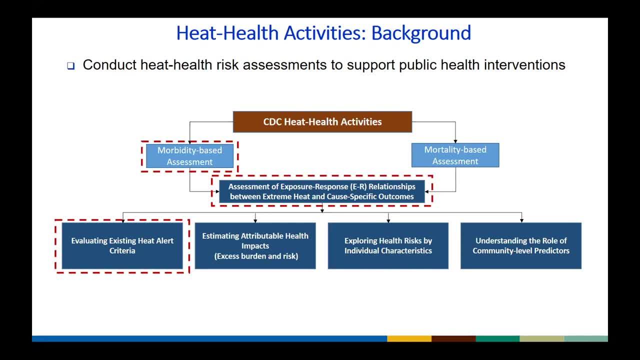 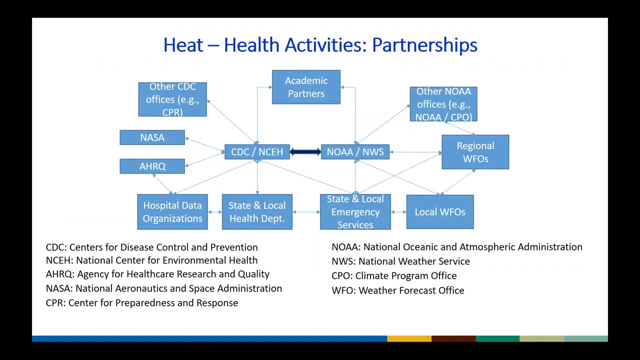 on morbidity-based assessments, primarily looking at how that evidence was used to inform existing heat alert criteria. And before I actually start discussing the data sources and methods, you know, I also wanted to sort of thank the partners involved in this project, Sort of. 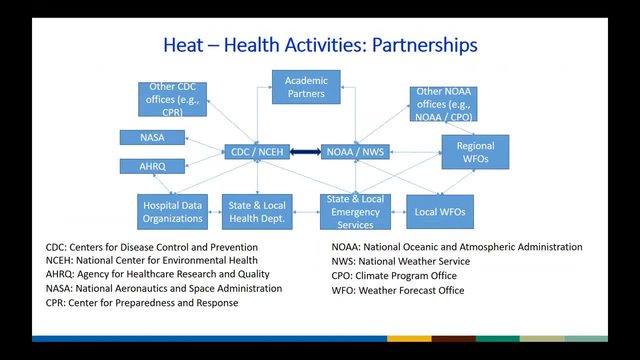 you know, we were able to leverage existing partnership and establish some new ones, and we're extremely thankful for the support provided by various organizations. And then this block diagram reflects various partners that were involved in the project, either as data stewards, subject matter experts. 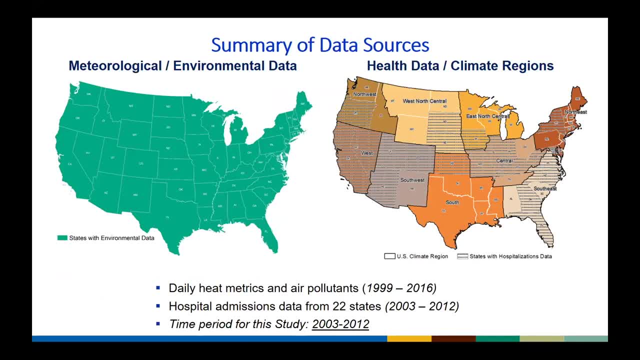 or as outras expert stakeholders. And in terms of data sources, we were able to put together a comprehensive research data set with a suite of daily heat metrics from both station and model-based data sources, and also coming up with long-term health data sets for hospital admissions. 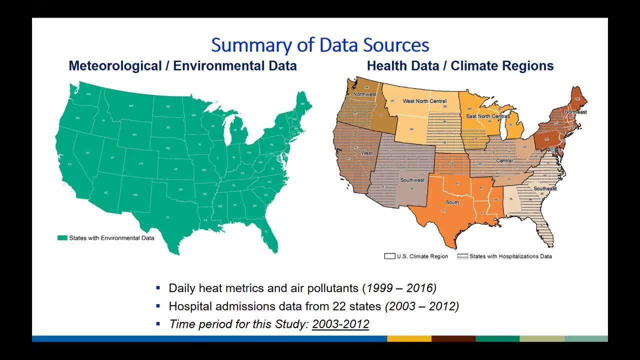 So, basically, the daily heat metric data we used for this project. we used a model-based data product from the North American Land Data Assimilation System, So these are gridded data products which were then converted to match county resolution, And then they're. 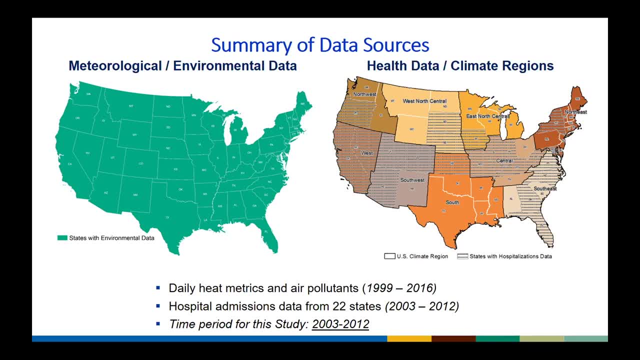 available for the lower 48 states And then for the hospital admission data. we had daily county-level health data from 22 states And the data came from Agency for Healthcare Research and Quality, And the database that we used from AHRQ was the state inpatient databases. 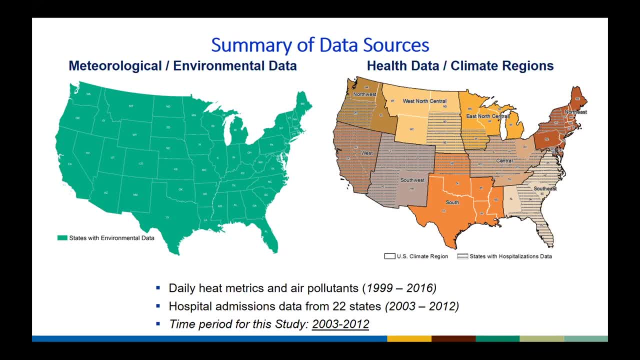 So the time period for the study, basically determined by the availability of health data, was 2003 to 2012,, which is like a substantially long 10-year time period. And then, before I move on, I also want to point out, like a majority of this analysis, 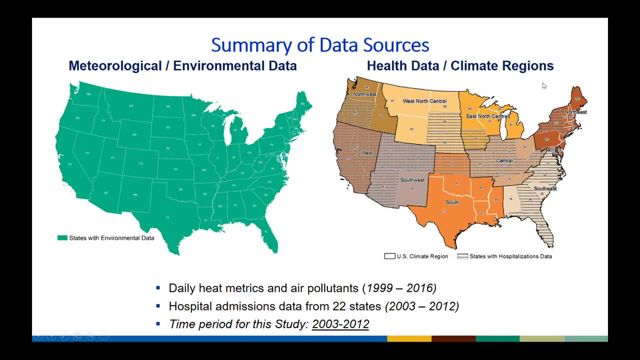 is either conducted by climate regions, which is something that NOAA uses and National Center for Environmental Information uses that, and then also by state, So you know be sort of highlighting sort of the work or the results that we got out of this project. 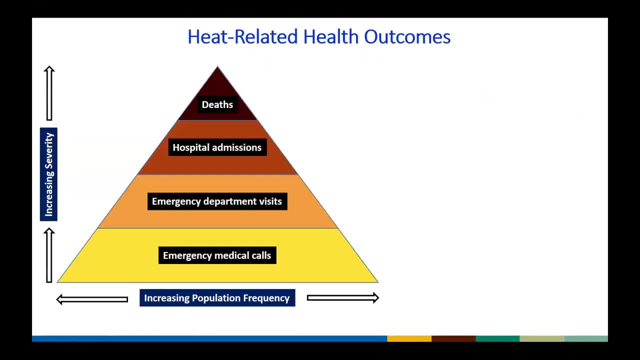 by both like climate regions and state. And then you're all familiar, I guess, like, with the heat-related health outcomes or the pyramid of health effects associated with heat. So, as you all know, like you know, a lot of studies have highlighted the impacts of heat. 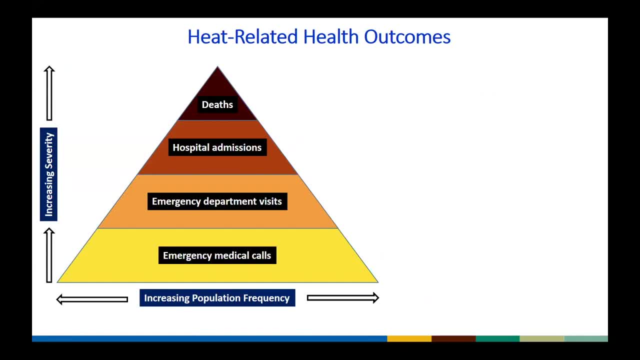 on any of this or all of these outcomes. But then we decided to go with something that's more specific, that's sort of not commonly attempted in health literature, where we're looking at hospital admission data but then also looking at certain cost-specific outcomes. So we looked at these various 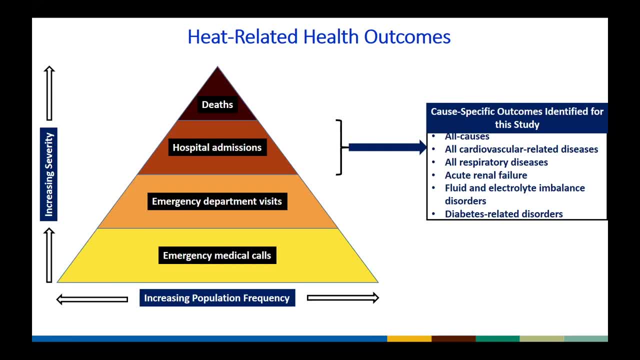 you know cost-specific hospital admissions in addition to all cost hospital admissions. So some of these may have. you know there's obviously existing scientific literature points to the. you know the impact of heat on these outcomes. But then we wanted to see how this sort 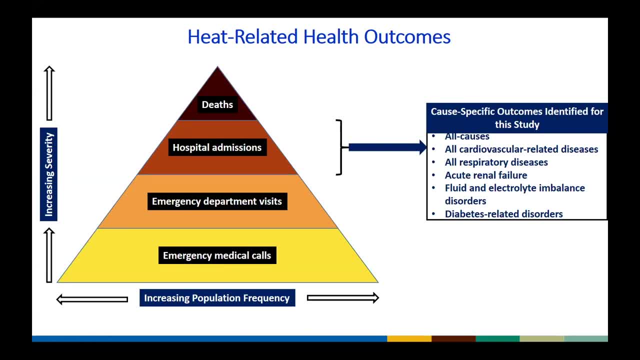 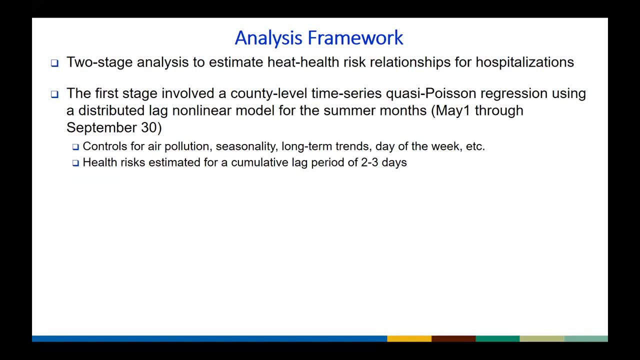 of varies across climate, regions, states and, you know, even across various subpopulations. And then, in terms of our analysis framework, we used a two-stage heat health- sorry, two-stage analysis- to estimate heat health-related relationships. So the first stage involved a 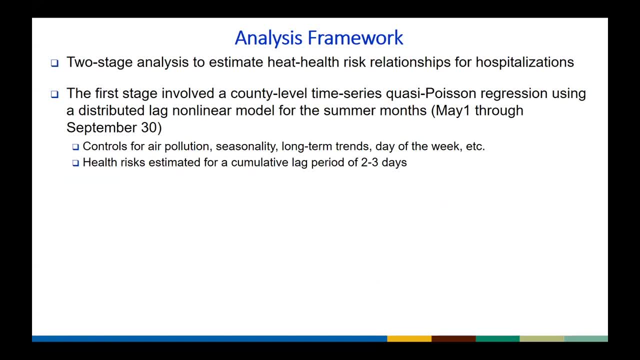 county-level time series, basically using a quasi-poison regression. And then, as Greg mentioned, we also used a distributed lag non-linear modeling framework. So our analysis was done for the summer months, for those 10-year time periods. And then the reason why we used the 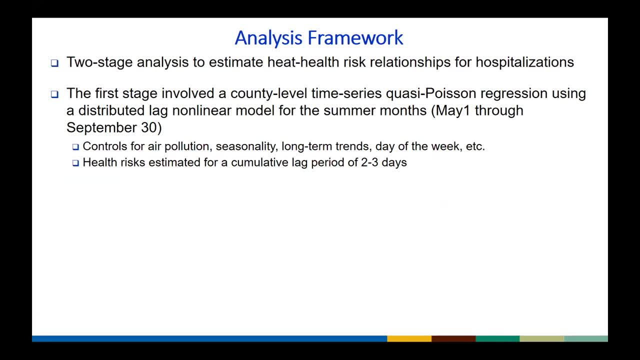 used a DLNM approach was so that we could explore non-linearity in the exposure response relationship as well, as you know, quantified delayed or extended effects in the lag dimension. so I think I thought we thought both were important. and then the second stage involved pooling of county level. 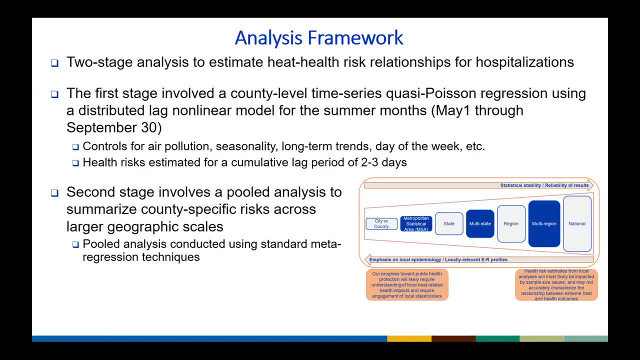 helpers from the first stage to generate, like stable exposure response profiles and then also measures of excess burden across these various geographic scales. and the graphic in the bottom right, you know, indicates sort of the trade-off that we face when we are conducting and presenting results at finer geographic scale versus, you know, generating results that are statistically. 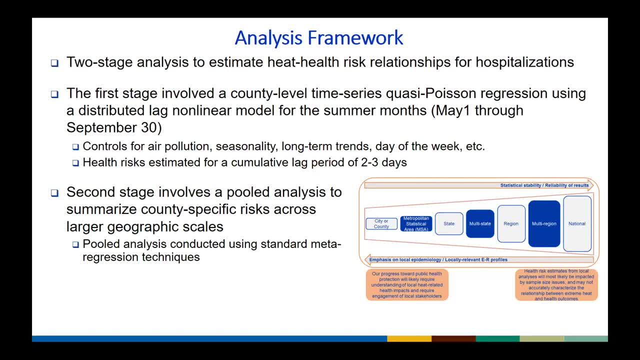 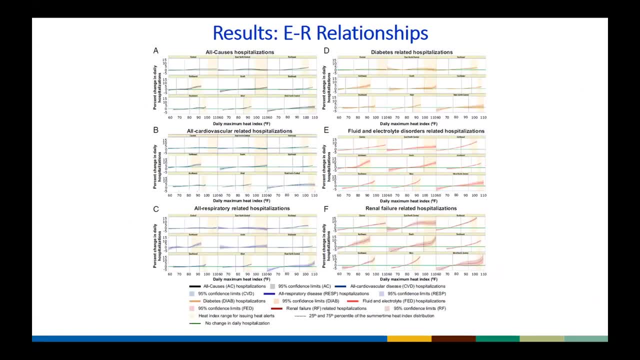 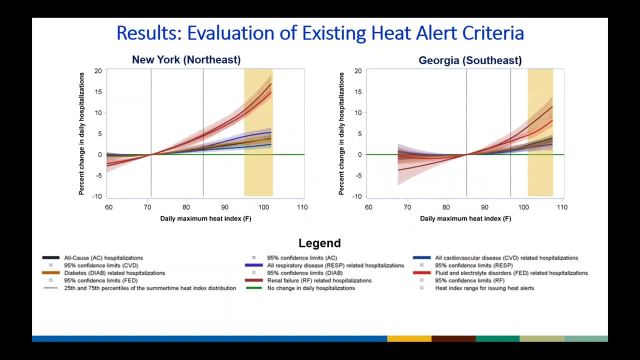 stable and reliable, something that's sort of needed for translating these research findings for a public health practice. and then this chart describes the region-specific exposure response relationships for various hospital admissions. again, like there's a lot to take in in this sort of presented in the manuscript, But if you sort of zoom into two different states, 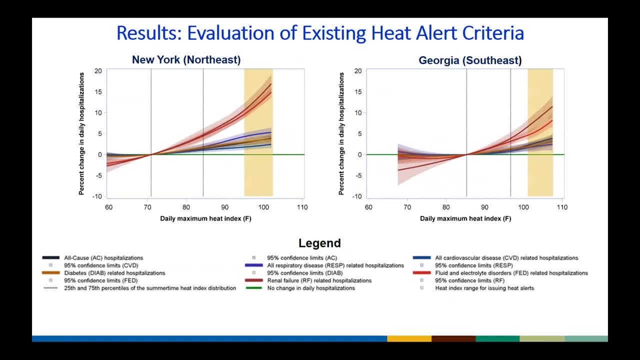 in those climate regions, say the northeast and the southeast climate region. so what you're seeing is sort of the increase in health risks as a function of daily maximum heat index. So, and these are for the various hospital admissions that you're looking at, 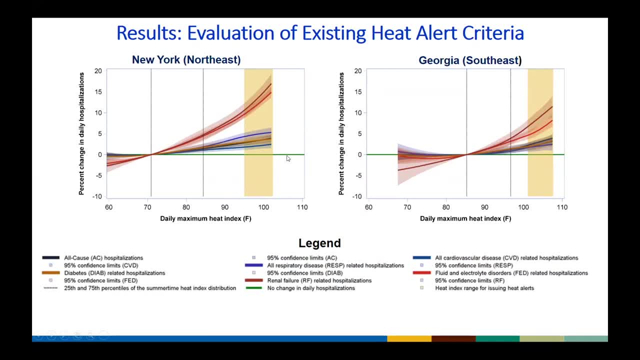 So these, obviously the green line here indicates no effect or null effect. And then these percentiles, like these vertical lines, indicate the 25th and the 75th percentile. So basically looking at the interquartile range, And then these bands, the golden, yellow or 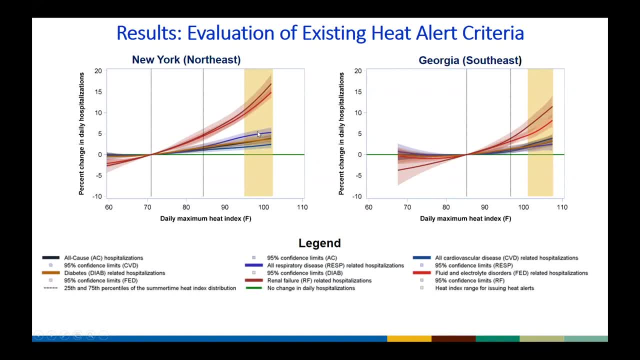 those bands here indicate typical alert temperatures that are used for, you know, issuing early warnings for heat. So, as you can see from both states, there is a disconnect between the- you know, the heat index ranges that are used for issuing alerts and where you start to see the increase in risk sensitivity to heat. 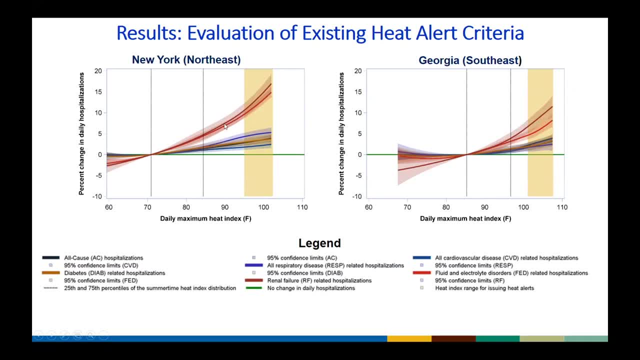 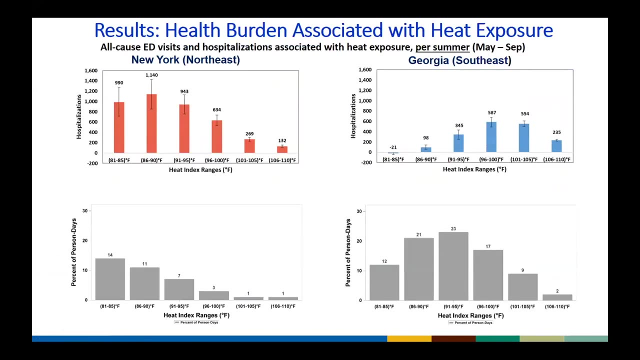 And some outcomes, for example the acute green hole failure and fluid and electrolyte imbalance, are sort of more sensitive compared to other more chronic outcomes. So again, like this, varies based on the slope, varies based on climate, regions And if you sort of translate the information that was presented as risk into excess burden. 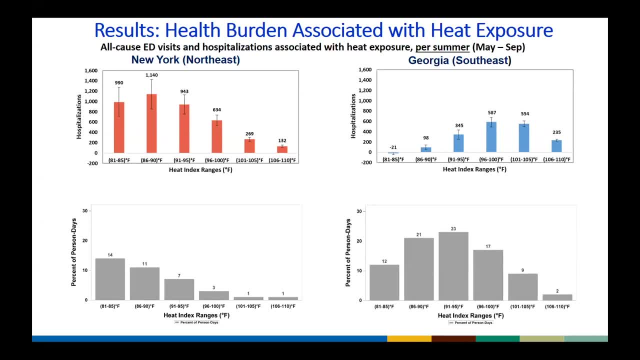 gain burden, which factors in sort of the first in base of exposure. what you see here is completely different, Like so, for example, in New York State, the burden that you notice is happening mostly in the moderately high heat index value. So by 95, you have almost like 60% to 70%. 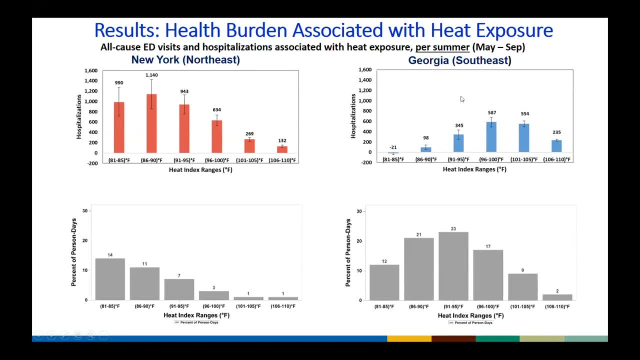 of all, the excess burden associated with heat happening versus, like in Georgia, it's sort of increasing when you hit like something like a 95 degree Fahrenheit for heat index. So again, like in this sort of mimics, the person days of exposure, like here. 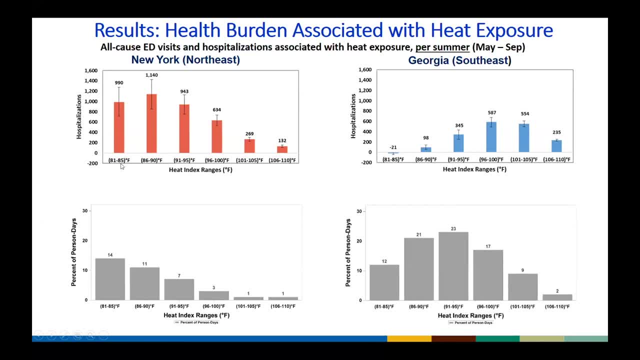 like in the bottom panels indicate sort of how prevalent those temperatures are in these various states. So, regardless of like how you like understand these relationship between burden as a function of person days of exposure, one thing we can notice is the alerts that are issued like in these states are fairly high. So, for example, in New York state you notice that the 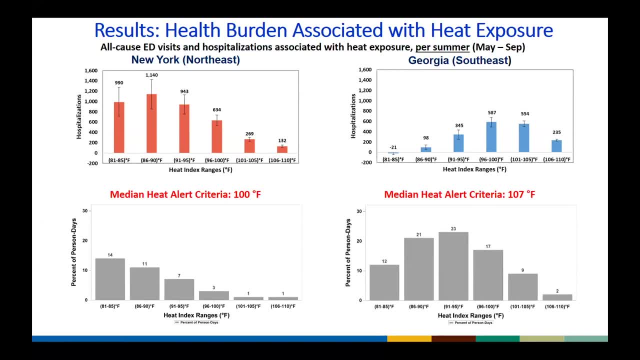 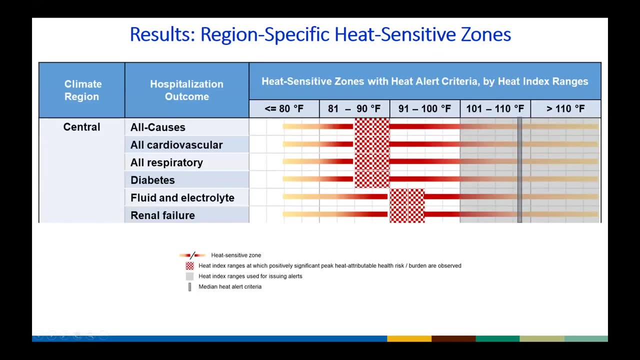 alerts are issued at 100 degrees Fahrenheit, and in Georgia it's even higher: it's at 107 degrees Fahrenheit. So and then off. note, like notice, that the majority of your health burden is occurring at somewhat moderately high heat index values. So what we did was we were able to. 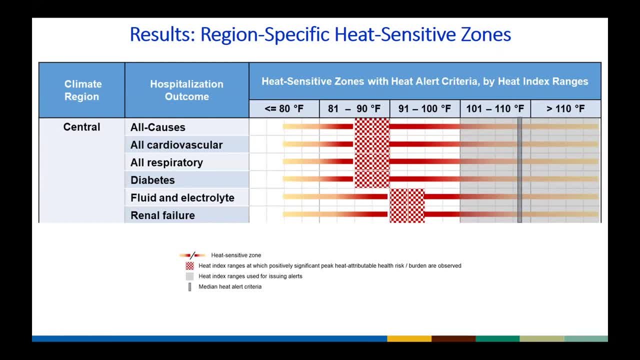 translate all this information, these measures of excess burden, and maybe like a game chart sort of looking at these risk and burden information in the context of sort of what the weather community might be interested in, sort of showing them where you start to see an increase in piggyasis, health impacts associated with heat. So these lines sort of. 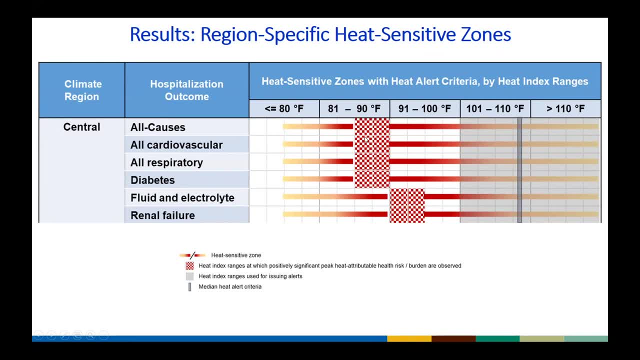 start to indicate where you tend to see sort of an increase in burden, significantly positive health burden, and then where it peaks, which is sort of indicated by these checkered boxes And then sort of all, Also the gray area and the vertical bar on the right. 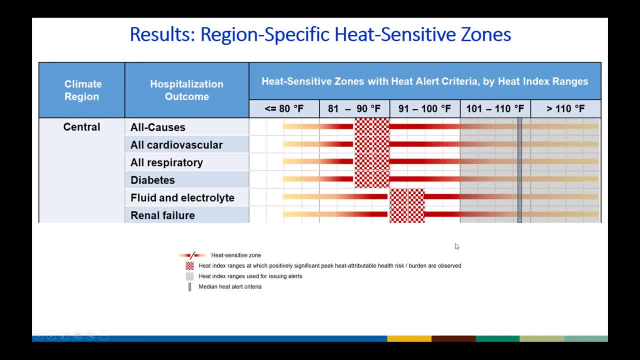 indicates where you typically see heat alerts being issued. So those are the heat index ranges where currently heat alerts are issued. So, again, our goal for this chart is to express the disconnect that sometimes you see in various climate regions between heat index ranges that are sensitive when it comes to health effects. 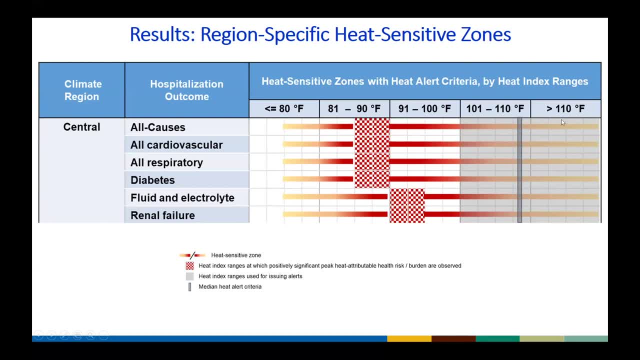 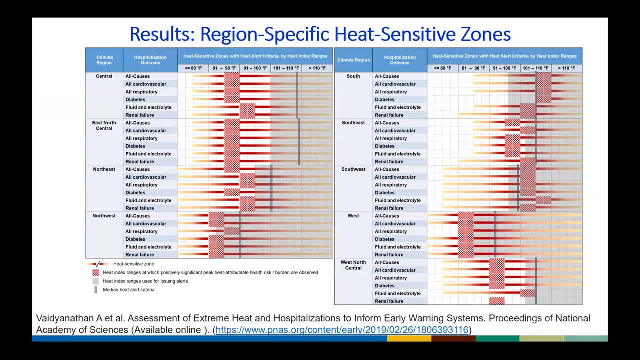 and heat index ranges that are associated or that are currently calibrated to be used in early warning systems. So what we did was we summarized all these relationships for every single climate region And then, in the appendix of the paper that was published, we also provide information by state. 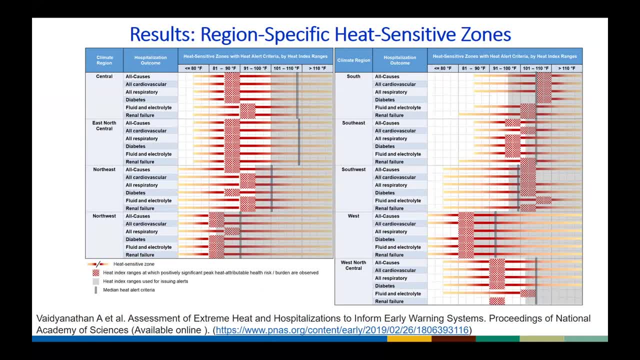 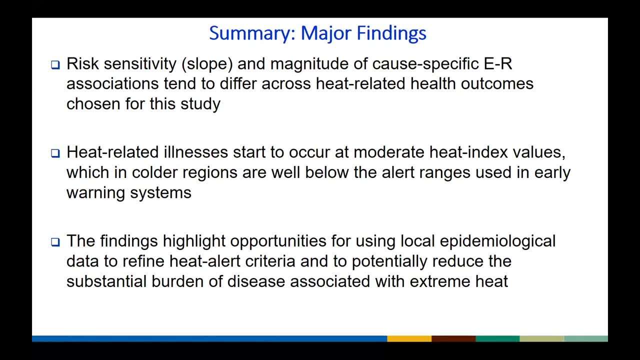 as to how these sensitive heat ranges vary by state within each climate region. I don't know if I have enough time, but I think we're about there, But the major findings here that we noticed in this study was the risk sensitivity or the slope. 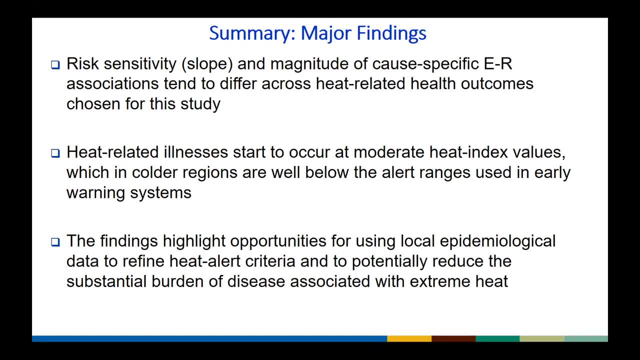 and the magnitude of all these cost-specific ER outcomes differ across heat-related health outcomes. That's one. Also, we noticed that relationship changes with climate regions. And then the next thing that was of interest to primarily the weather community was we started to sort of point out: 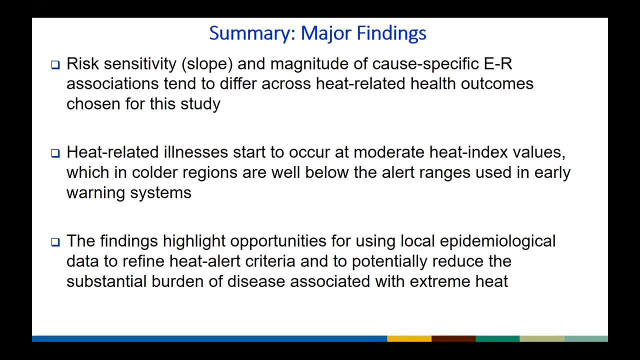 even at moderately high heat index values, say in colder regions, we started to see heat-related burden And then also comparing that against all the alert ranges used for early warning systems, it sort of expressed sort of the discordance between what's being used for heat alerts versus where. 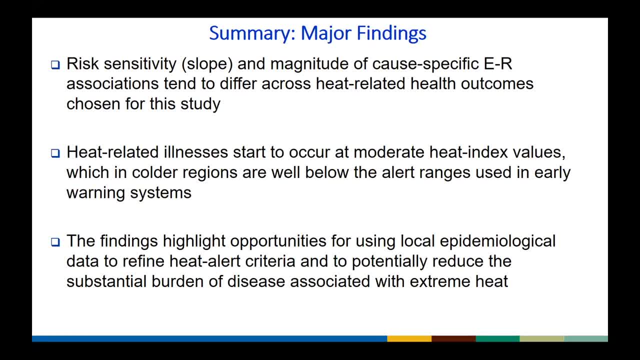 those ranges that are sensitive from a public health standpoint And then also personally. it was very interesting for us to use these local epidemiological data to refine heat alert criteria and also to explore how the burden associated with heat varies across a wide spectrum of heat index ranges. 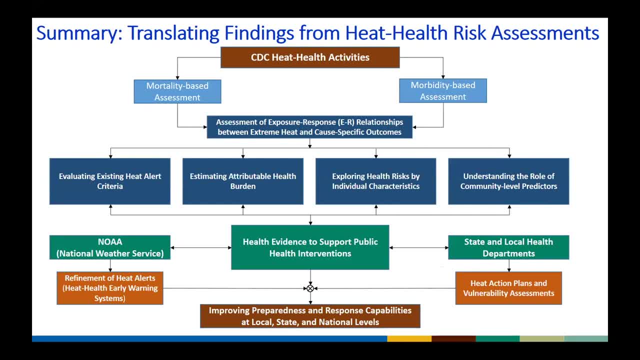 And so this is sort of a summary of what we intend to do with this effort. So I guess you've seen sort of the aspect that is related to evaluating existing heat alert criteria and then how we're sort of sharing this information with National Weather Service. 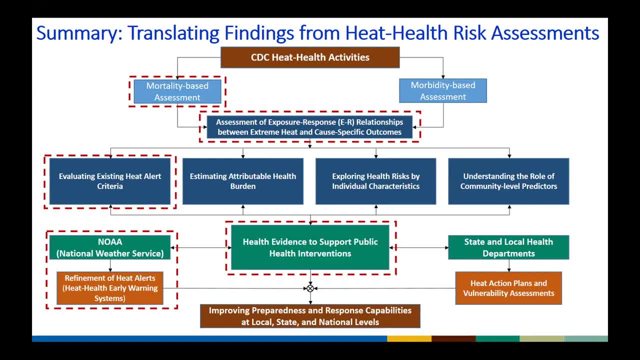 And then our current work with refinement of these heat alerts. But there's also other aspects that we want to complete and which we're doing, which are ongoing projects. So basically we want to sort of look at burden now which will basically improve our preparedness and response. 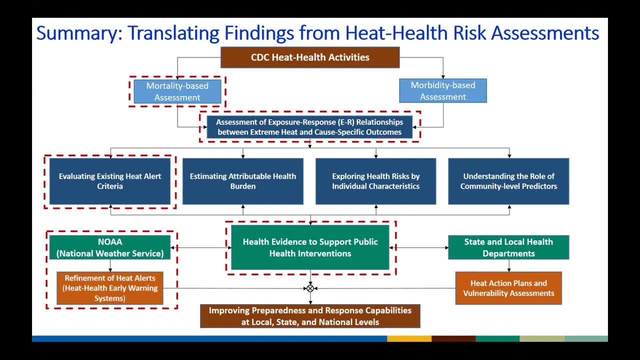 capabilities and then also use this information in a climate context. For example, we would be able to use this information and project burden in a future climate scenario or looking at various climate scenarios and understanding how these exposure response relationships change. So that's something that we're also planning to do. 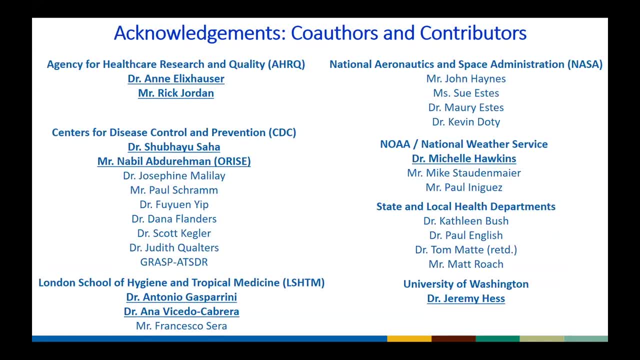 And then, before I want to conclude, I want to really thank all my co-authors. It was great to work with my co-authors whose names are underlined in this presentation. I feel very fortunate to have received great input and support from them. 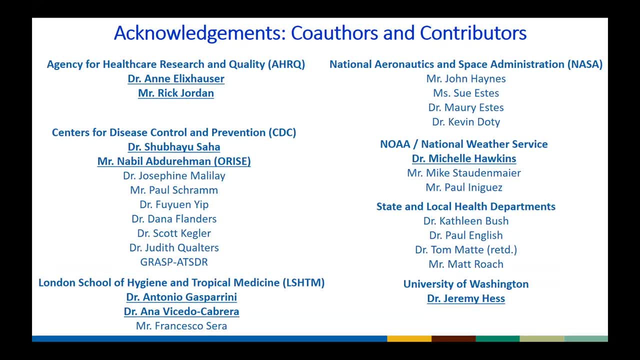 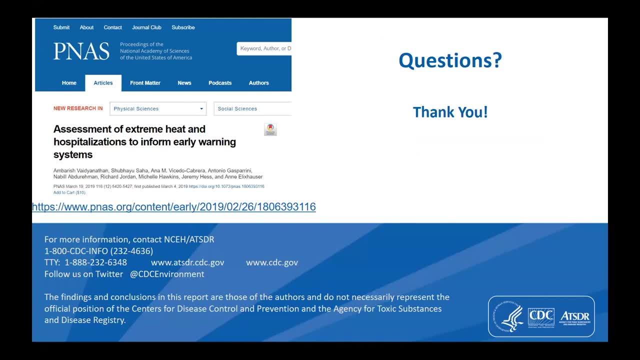 And I also want to thank other contributors who provided scientific and or programmatic support for this project. And lastly, here is a link to the article that I've mentioned. I think it's available from the webinar page And then also, it's perfect timing for us. 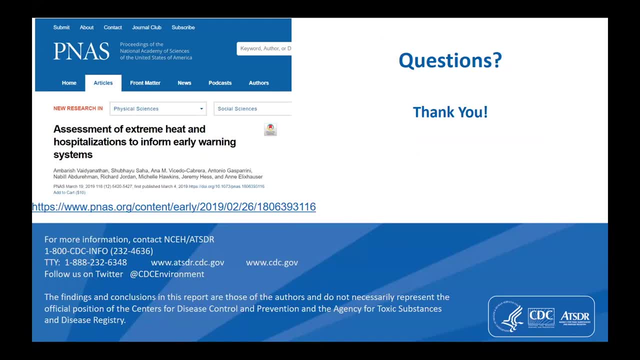 to get this article out, because I work for the climate health program at CDC and then we're celebrating our 10th anniversary, So perfect timing With that. any questions? Thank you Great. Thank you, Dr Vadhyanathan, for your presentation. 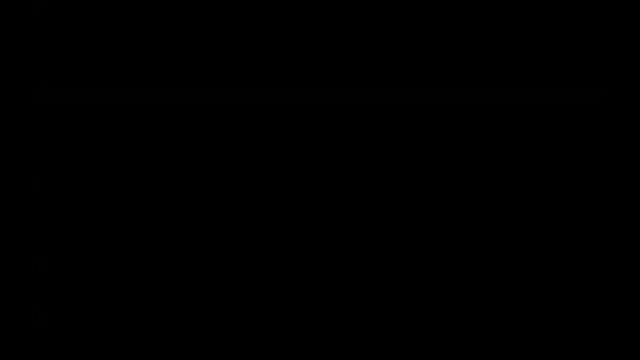 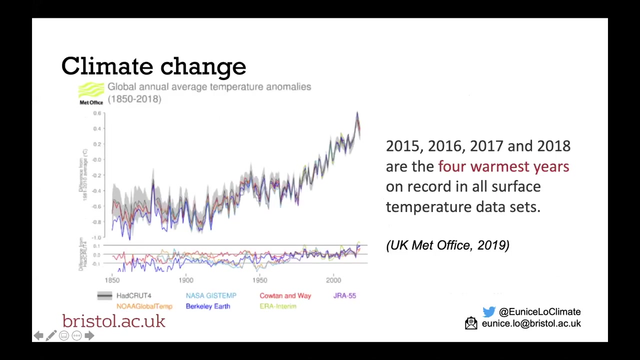 We're going to move into our last presentation with Dr Lowe, who's going to discuss her work, And while we're switching over, just let me remind you that there is a Q&A box for you to enter your questions so we can get to them at the end. 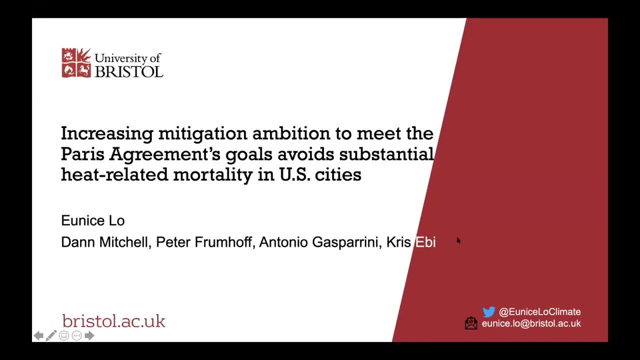 Thanks, Yeah, can you hear me? Yes, Yeah, so hello, I'm Eunice Lowe. I am a climate scientist, So it's a difference. I have a different background to the previous two speakers, which is great, because this session is. 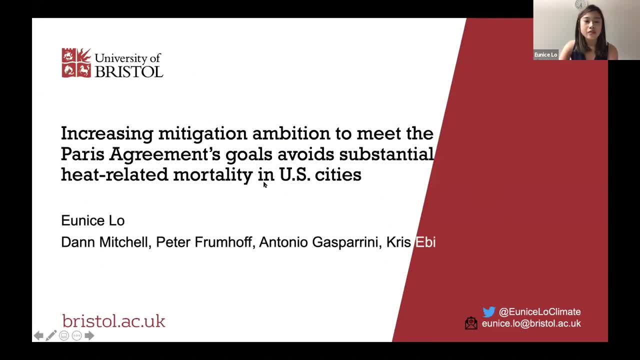 about climate change and health, So I'm going to talk about a paper that I published a few months ago, which is about how increasing mitigation ambition to meet the Paris Agreement's temperature goals could avoid substantial heat-related mortality in cities in the United States. 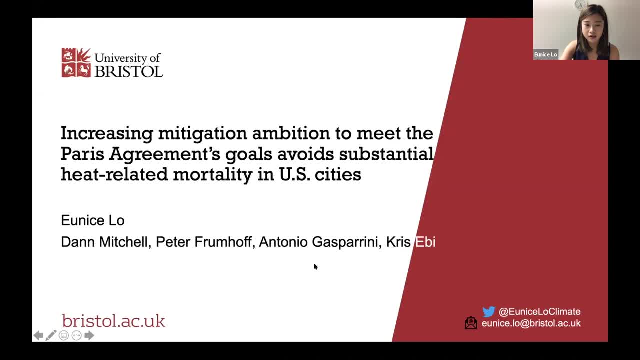 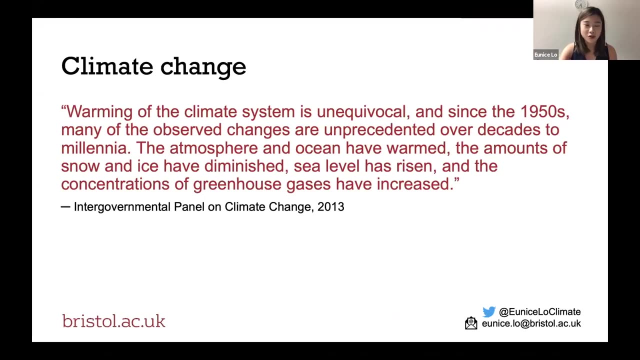 I just wanted to start the talk by actually talking about climate change. This is a sentence taken from the fifth assessments report from the Intergovernmental Panel on Climate Change from six years ago, and back then we already knew that warming of the climate system is unequivocal, and since the 1950s, 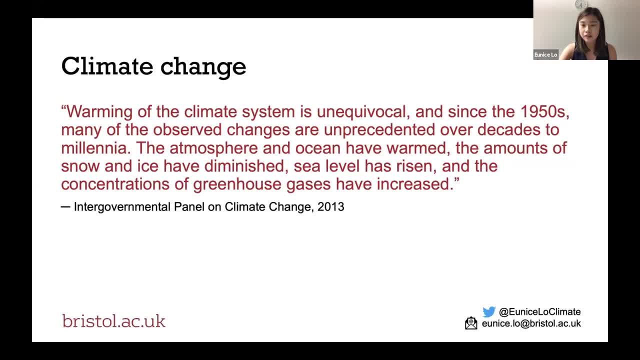 many of the observed changes are unprecedented over decades to millennia. The atmosphere and ocean have both warmed, the amounts of snow and ice have diminished, sea level has risen and the concentrations of greenhouse gases have increased. Especially for the observed increases in temperatures, we are quite, very confident that it can be attributed to human influences on the. 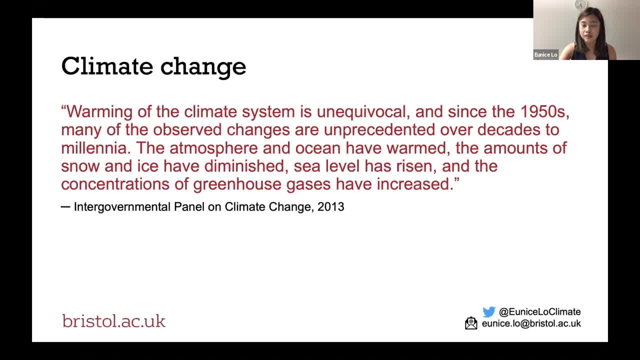 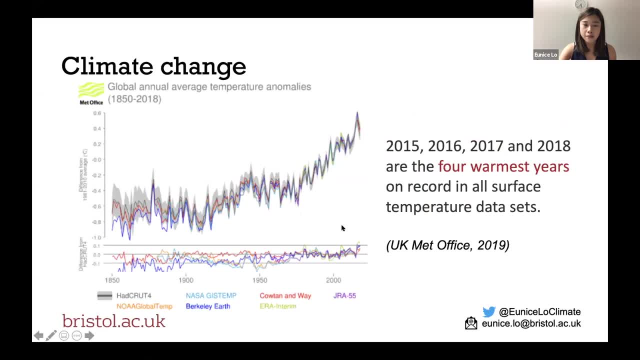 climate, ie human emissions of greenhouse gases, including carbon dioxide. This is a graph taken from the UK касmet's office and it shows the global average temperature from 1850 up to 2018.. 1850 on the left and 2018 recent years on the right here and we can see that the global average 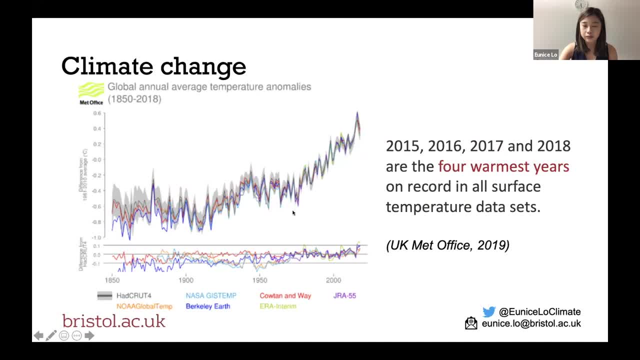 temperature has definitely increased throughout this period of time and in fact the last four years are also the four warmest years on record in all surface temperature data sets from around the world. so this graph here have different, has different colors and they show data from different national. 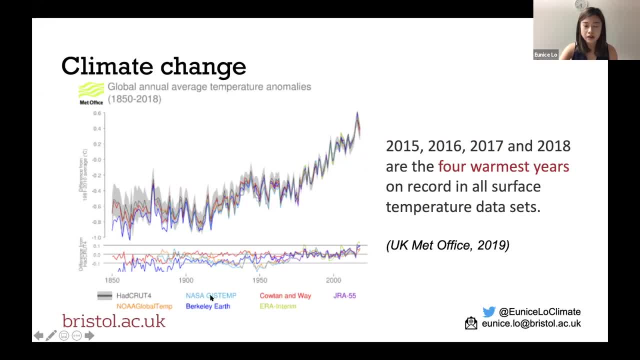 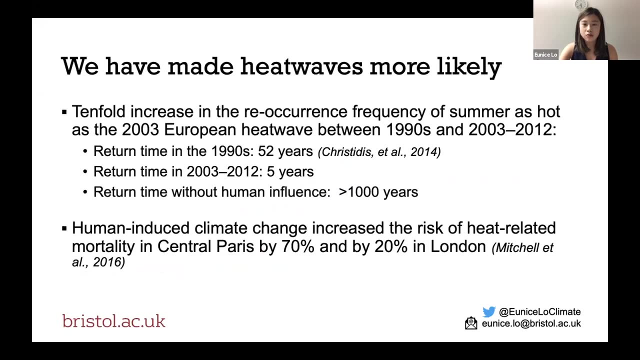 agencies from around the world, including the UK, US, European, Europe and also Japan, and they all agree that the last four years were the warmest four years on record. so not only have we increased global average temperatures, we as humans have also made heat waves more likely, and so a lot of studies have. 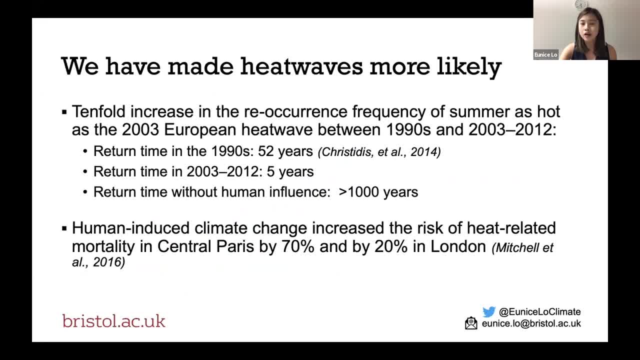 looked at the 2003 European heat wave, where maximum temperatures were above 40 degrees Celsius in many parts of Europe, including France, and so one study found that there was a tenfold increase in the reoccurrence frequency of a summer that is as hot as the 2003 European heat wave, just between the decade in the 1990s and. 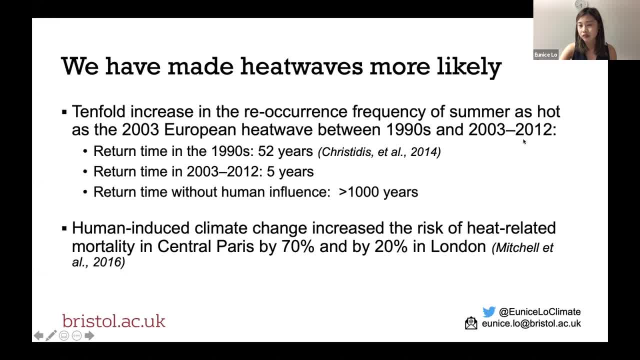 a decade in the early 2000s, which is two years ago, and the last four years were about the same as the 2000s, which is 2003 to 2012. so in conditions in the 1990s such a heat wave with would have happened about one in 52 years once. 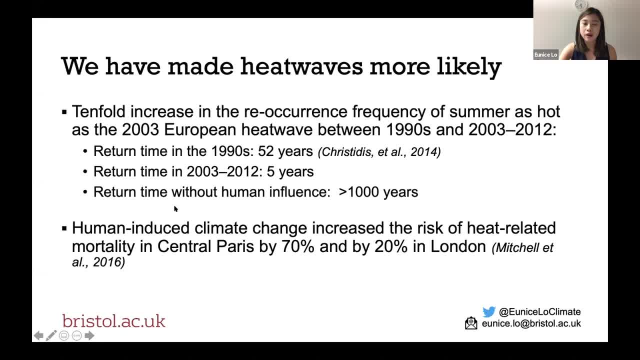 every 52 years, but in the decade in 2003 to 2012, the this heat wave would only have happened once every five years. so there was a ten, ten ten fold increase in the probability of such an event, and just from the 1990s to the early 2000s. 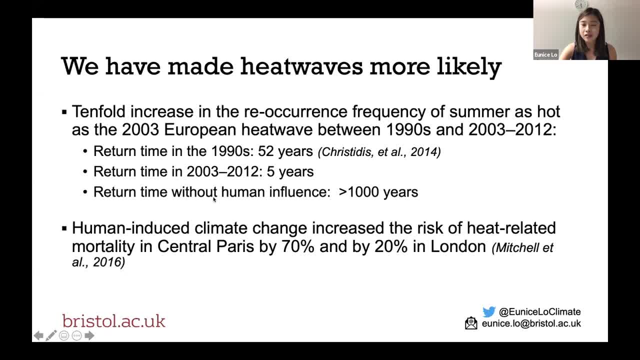 and in a world that doesn't have any human influence, then such a heat wave, which only happened once every over thousand years, and so many people unfortunately died during the heat wave and I think heat related deaths were over 700 in Paris and over 300 in Greater London, one study in London and one study in London that was found to have a very high chance of death. 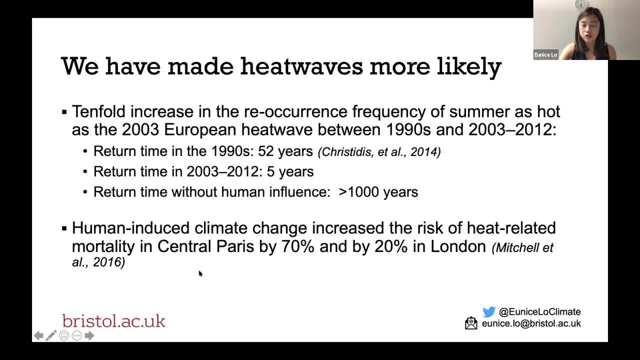 2016 found that human-induced climate change has increased the risk of heat-related mortality in central Paris by 70 percent and in London by 20 percent. So we have made global temperatures to rise, we have made heat waves more likely and we have also increased the risk of heat-related 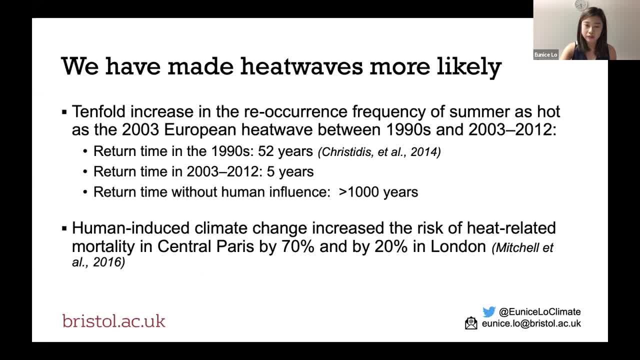 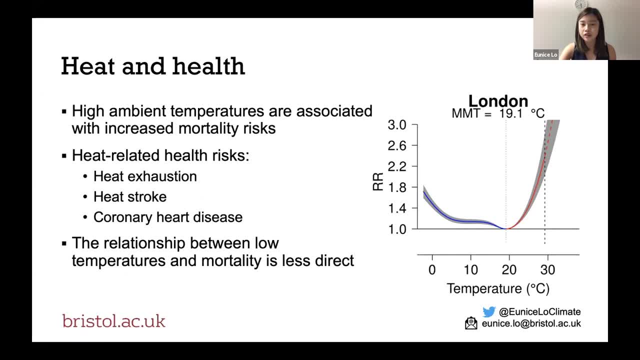 mortality in some deadly historical heat waves, And that's because high-ambience temperatures are usually associated with increased mortality risks. So, similar to the previous two talks, this is an exposure-response relationship between temperature and mortality for London, found from a distributed lag nonlinear model with historical data. So for London we can see: 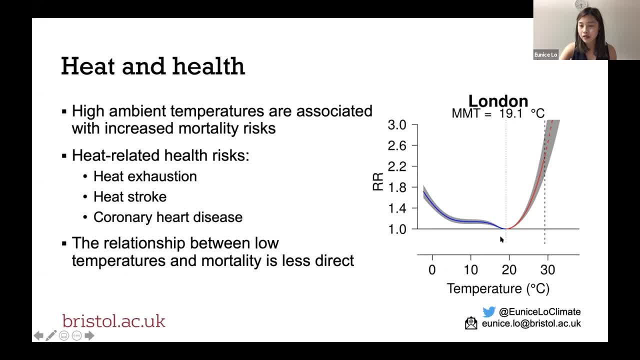 the lowest mortality risk happens at around 19.1 degrees Celsius, and any temperatures higher than this threshold are associated with an increase in mortality risk, And common heat-related health risks include heat exhaustion, heat stroke, which can be a medical emergency, and also heart disease. 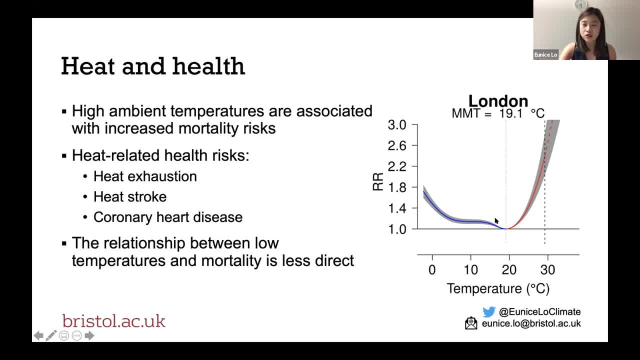 But we have less confidence in the relationship or the direct risk of heat, which can be higher. so for the first two reports we have more confidence in the relationship between lower temperatures, which is the blue curve here, and mortality. So in this talk and 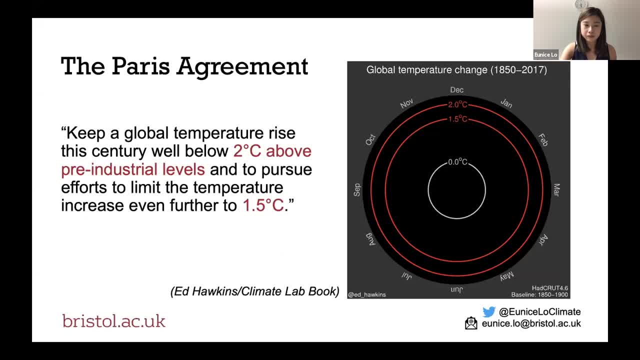 in this paper, we focus on the heat side of this curve, which we have more confidence about. So, with all that, knowing that climate change has adverse impacts on human health, and also if we fear in the future, so we have these international agreements of the climate in paris, called the. 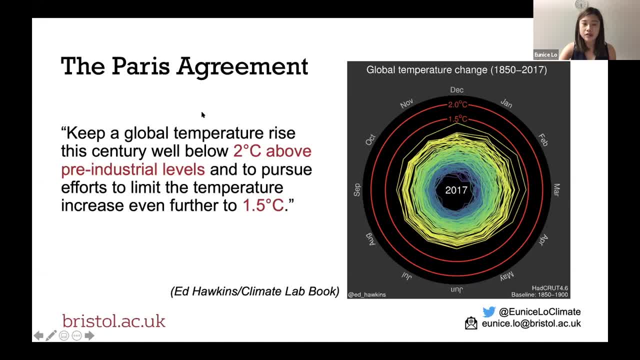 paris agreement, and the main goal of these agreements is to keep a global temperature rise this century to well below two degrees above pre-industrial levels and to pursue efforts to limit the temperature increase even further to one and a half degrees um. on the right here i'm 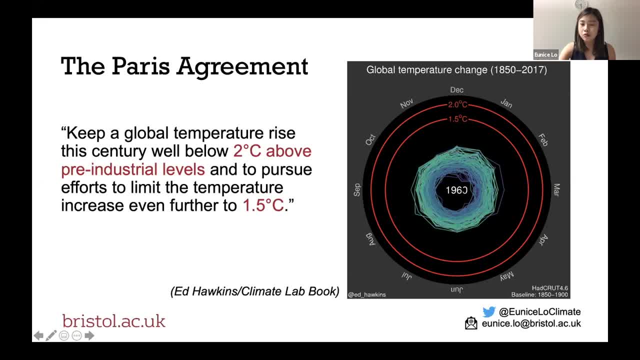 showing an animation by ed hawkins, and so it shows how temperature- global average temperature- has evolved through time. so if we look at it again, in the middle is no temperature increase, so that's zero degrees above pre-industrial levels. these are the two paris agreements. 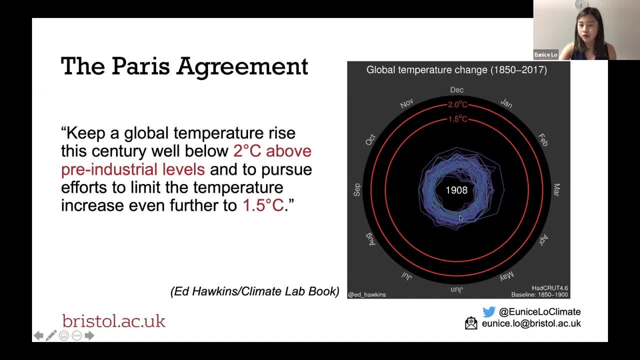 limits, and from 1850 up to 2017, we see these temperatures spiraling outwards, so closer and closer to the paris agreement's targets. and in recent years- 2017 and 2018- we are about one globally one degrees celsius above pre-industrial levels already. so we only have half a degree um to go if we want to limit. 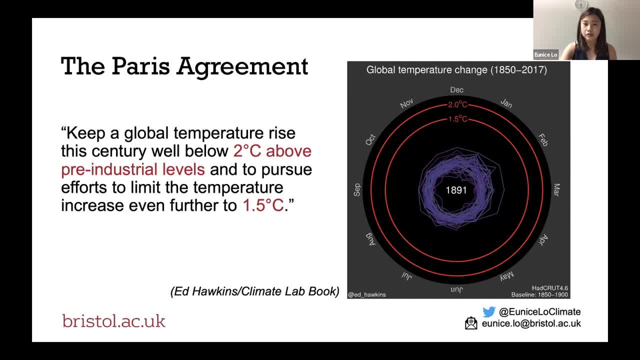 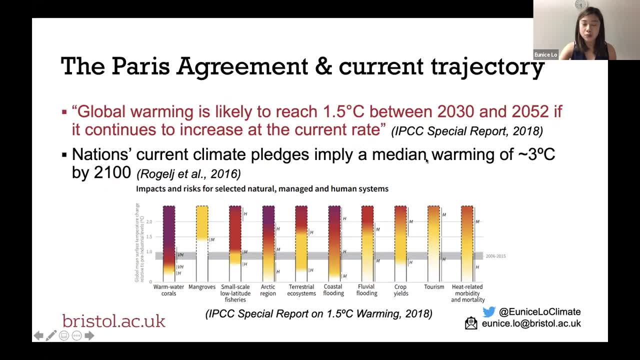 global warming to one and a half degrees, according to the paris agreement. so here's a sentence taken from the um international agreement of the paris agreement. the paris agreement is a global warming agreement and the paris agreement is an intergovernmental panel on climate change special reports on one and a half degree warming. um, if global warming was to continue to increase, 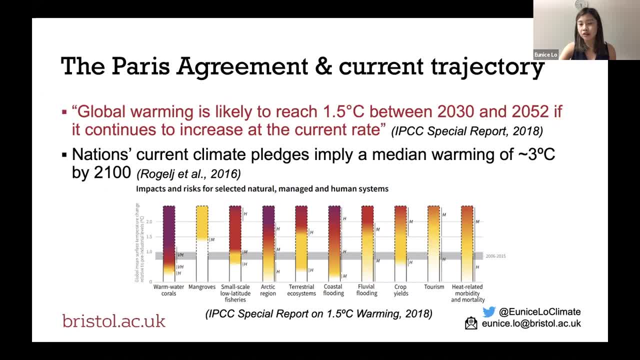 as the current rate, we are likely to reach one and a half degrees between 2030 and 2052, so the window of opportunity to mitigate more is closing really fast. um and also nations that are within the paris agreement, which is most nations in the world, um have put in a lot of effort to mitigate. 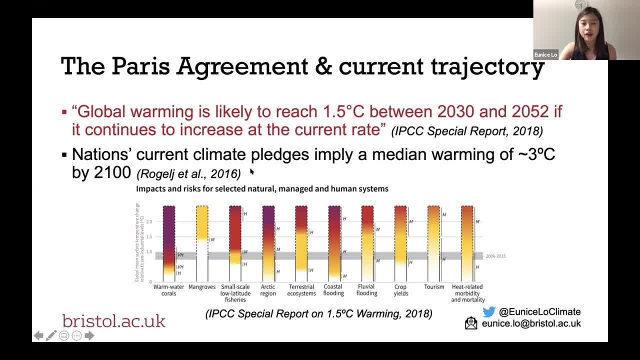 the climate change. and then, uh, we're able to see that the global warming is not less than two degrees more than the paris agreement. the conditions have changed in the environment by putting climate pledges um to outline the intended climate action for the future. but even if these climate pledges are all fulfilled, or if the unconditional pledges at least, 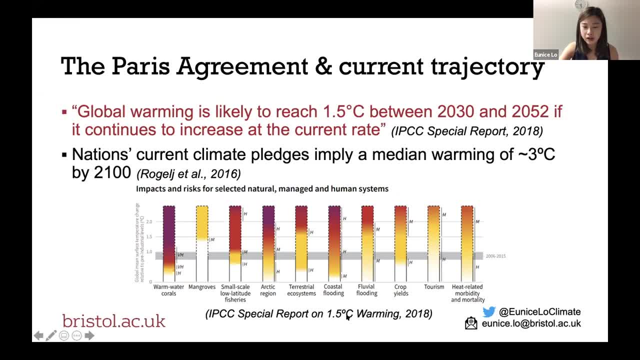 are all fulfilled, then and if they don't change so they don't increase in the future, then once they found that the medium, the median estimates of global warming will still be three degrees above pre-industrial levels, so higher than the para schools. So this graph here is from the IPCC one and a half degree report I just want to highlight. 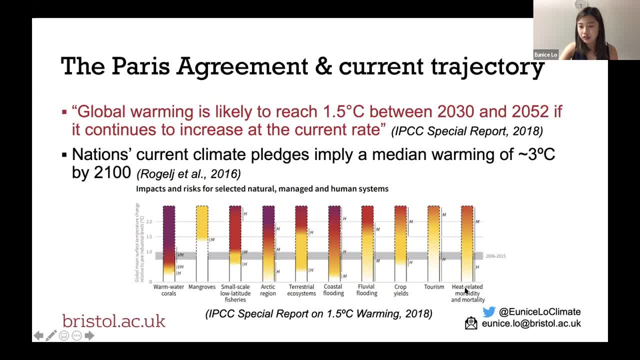 the last, the bar on the right here, which is about heat related morbidity and mortality. So currently 2006 to 2015 is about one degree warmer than pre-industrial levels. That is the grey horizontal bar here As temperature goes up, so moving upwards in the vertical direction. 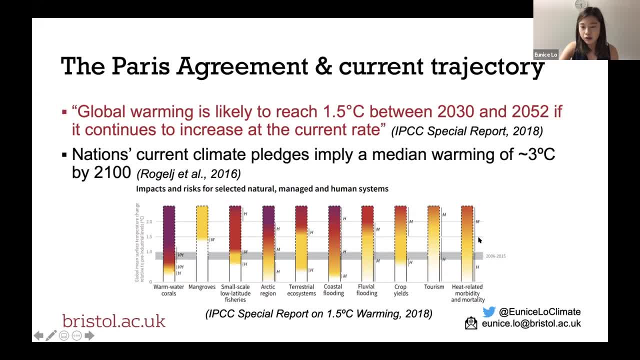 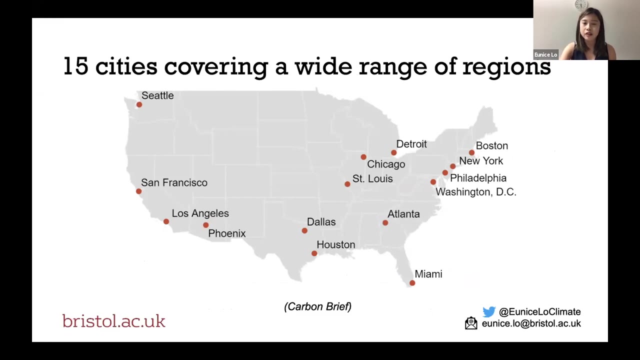 then it goes beyond one and a half and two degrees And the impacts on heat related mortality and morbidity is getting more severe and more detectable, as indicated by the colour change, orange and red being more severe impacts. So with all that background, what I did in my study was to look at the heat related 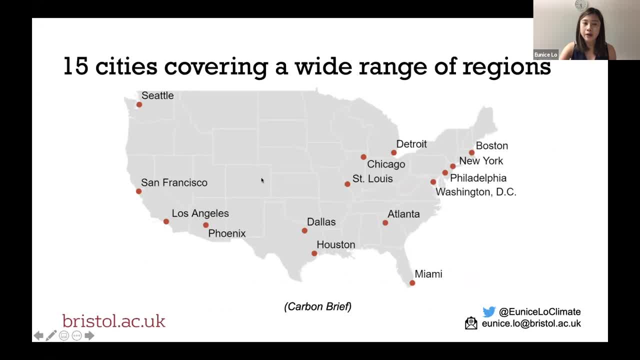 mortality levels On a city level in 15 cities in the United States in different future warming scenarios. So I have a scenario of one and a half degree warming, which is the more ambitious targets of Paris agreements. I have another scenario of two degree warming and I've also a scenario of 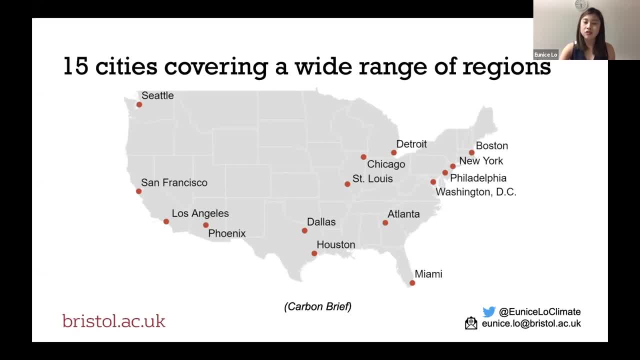 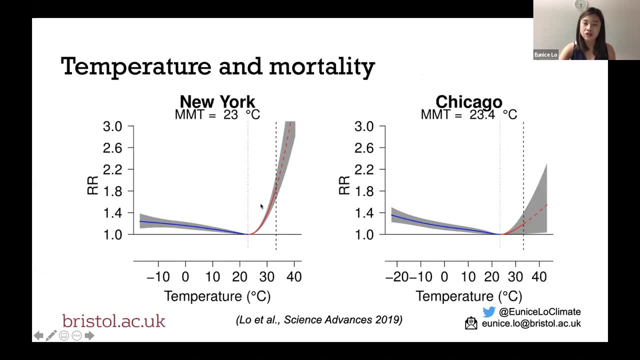 three degrees warming, about pre-industrial levels, And I wanted to compare the heat related mortality in each city in, you know, between these scenarios. So, first of all, what I did was that I found the present day relationship between temperature and mortality for all different cities, using observed data from, I think, 1987 to year 2000.. And these 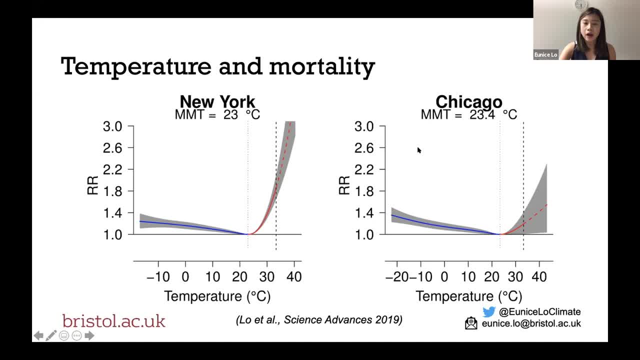 are two examples for New York and Chicago And, as you can see, above the optimal temperature, which for both of them is around 23 degrees Celsius, and there's a substantial increase in relative risk of mortality associated with higher temperatures. There is a dashed part dashed line in the red area on both of these graphs because in the 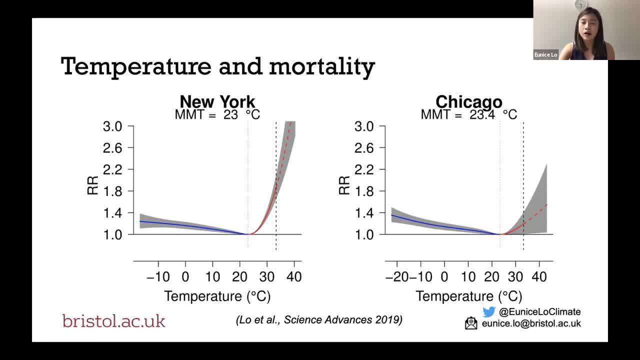 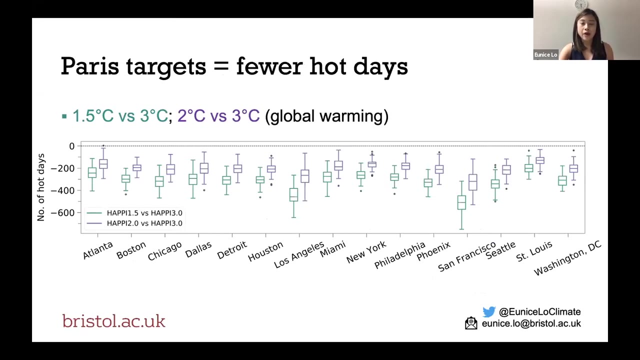 future under global warming. we're projecting even warmer temperatures that are unprecedented. So our data can't show us what the relationship between temperature and mortality would be from the observations. So the dashed parts of these graphs all come from from the existing data. So first of all, I have different climate scenarios. 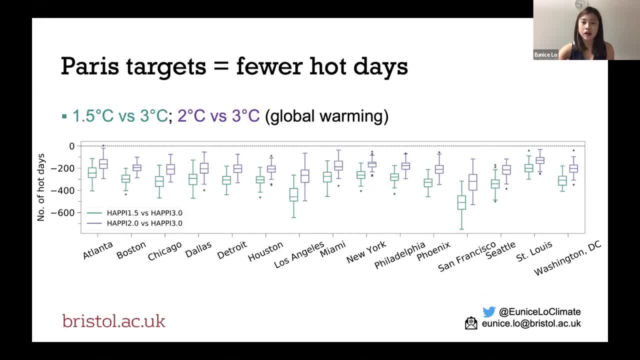 and I run these scenarios in different in decadal periods. So each run climate simulation is 10 year long and I counted how many number of warm days there would be in each scenario. So in this study I use the three degree scenario as the baseline because this is probably 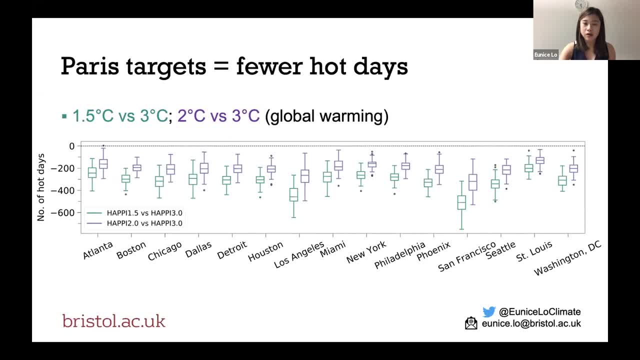 where we are headed, given the current national and international climate pledges, And so this graph here shows the number of hot days in a one and a half degree world compared to a three degree world, in green color, and in a two degree world compared to a three degree. 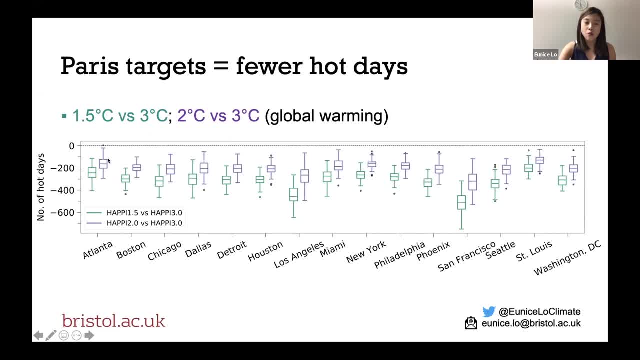 baseline in purple color. So they all have negative numbers, meaning that the models are suggesting a reduction in the number of hot days in basically all of these cities, in both the one and a half and two degree worlds, compared to the three degree world. But as you can see the green bars or the green ranges, 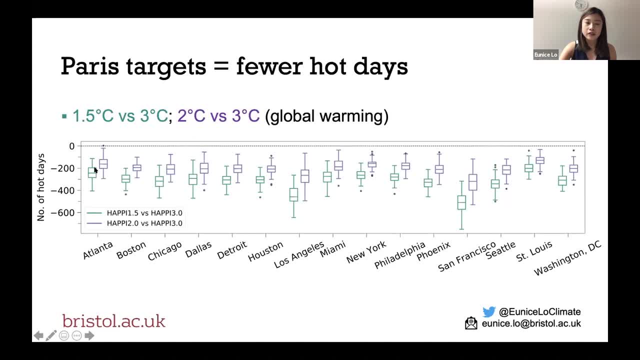 are even lower than the purple ones, Meaning that if we manage to mitigate to the one and a half degree targets, then we will expect more reduction, So fewer warm days per decade in all of these cities, even compared to the other targets, which is the two degree targets. 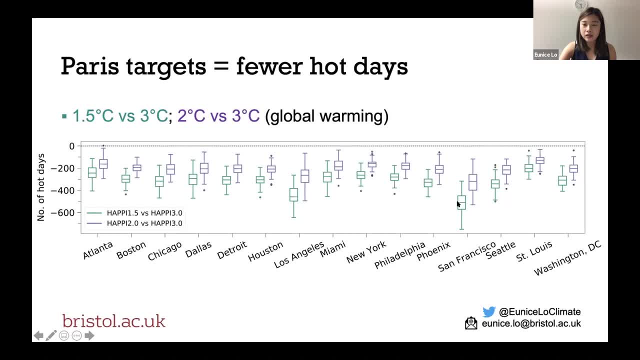 So if you look at San Francisco here, the median estimates of the reduction in the number of hot days in a one and a half degree world could be about 500 days per decade. So that translates to more than a year worth of days every 10 years. that could turn from a warm day. 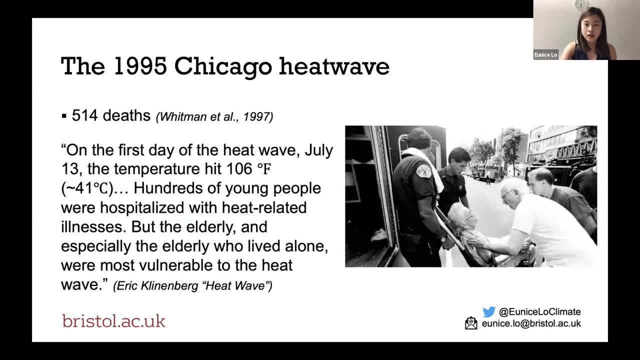 to being a cool day. So one of the results that I found was to compare the return times of heat-related mortality in a historical heat wave. So in the 1995 Chicago heat wave there were 514 deaths and temperature was up to 41 degrees Celsius on some of the days. 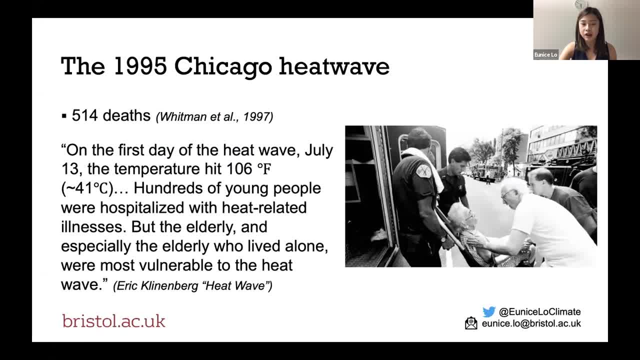 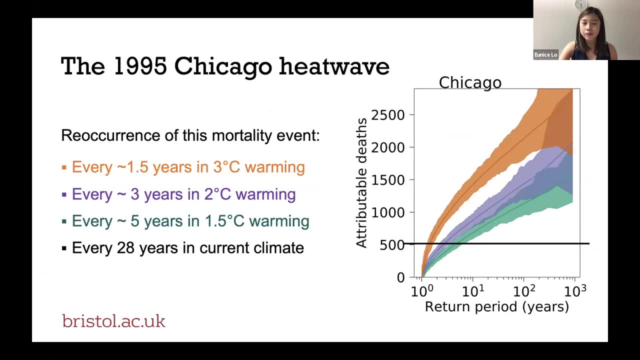 and hundreds of young people were hospitalized With heat-related illnesses. the elderly also suffered a lot. So 514 deaths happened during that event. So if we look at what are the reoccurrence probabilities of such a mortality events in different worlds under current climates? 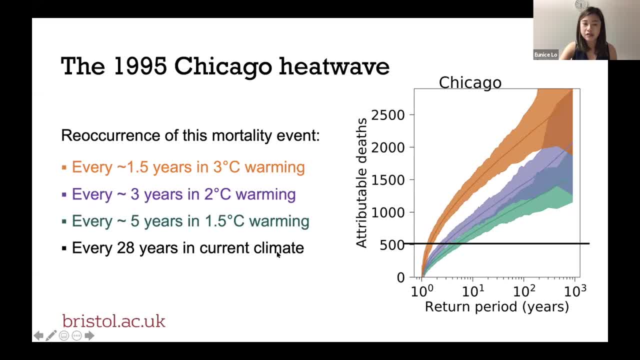 which is, I think, 2006 to 2015,, so relatively recent, having 515 deaths. sorry, 514 heat-related deaths would only happen once every 28 years, So relatively rare. But if global warming reaches one and a half degrees above pre-industrial levels, 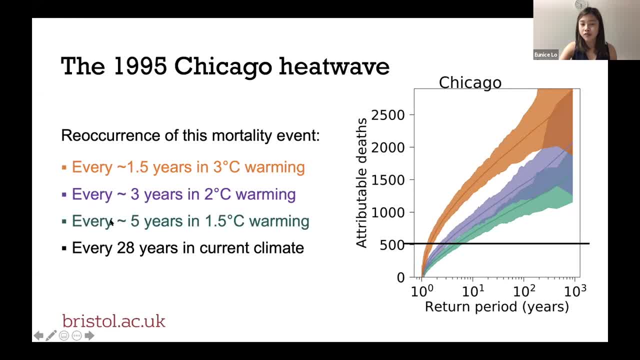 the probability of such a mortality events would become once every about five years, So a lot more likely, a lot more frequent. In a two degree world, this would be even more likely. These mortality events of 514 deaths would happen once every about five years. 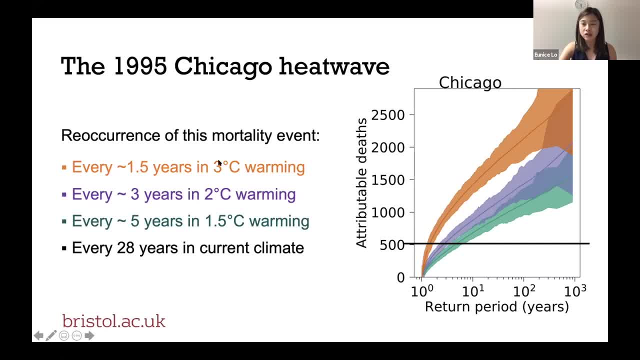 And if we go up to three degrees warming, which is actually what our current climate pledges are suggesting, then we are kind of expecting 514 heat-related deaths once every one and a half years. But I have to say that these differences in heat-related deaths across the scenarios 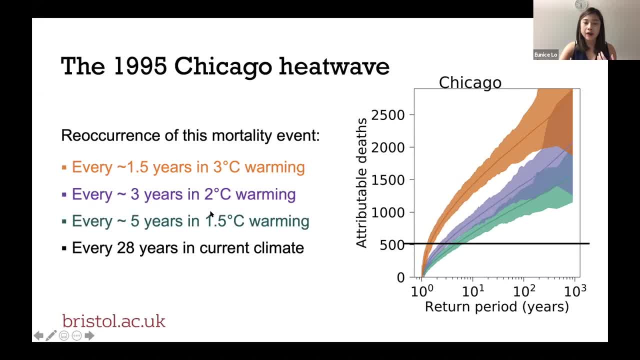 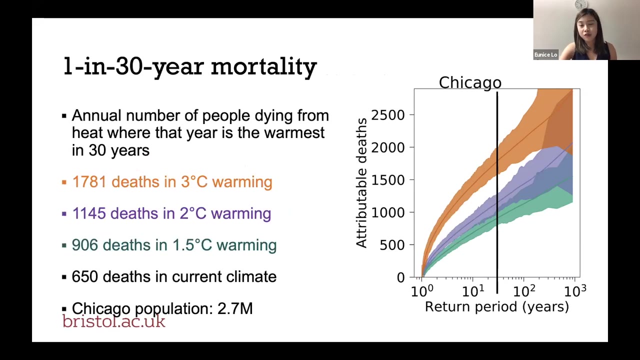 are only due to global warming, So I'm not accounting for potential adaptation or population changes as the globe warms. So we are isolating the impacts of rising rises in global average temperature on heat-related mortality in different cities. So another way of looking at this: return period curve. 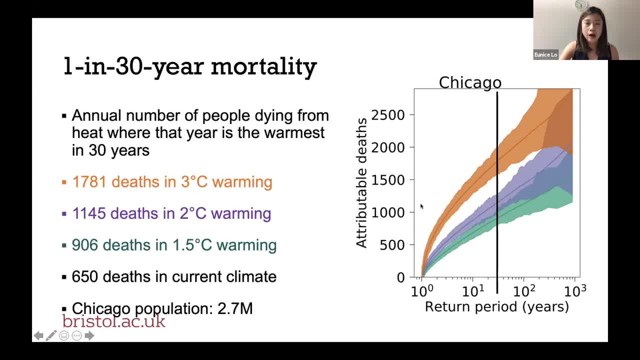 which is very common in attribution studies is to look at a certain rarity of an event. So I've chosen an extreme event being defined by its coming back once every 30 years. So is this vertical line here? So all intersections with this vertical line. 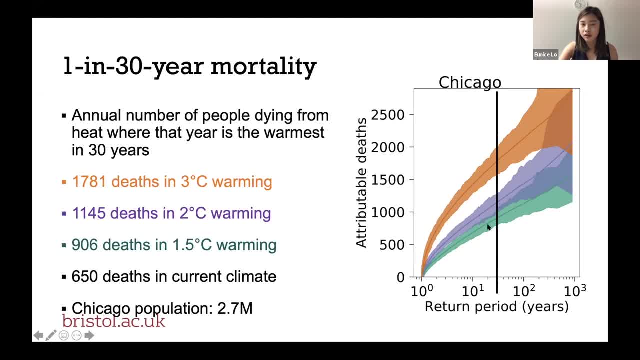 will give me the number of deaths related to a one in 30-year heat event in different worlds. So in current climates, once every 30 years we expect 650 deaths In a one and a half degree warmer world- a one in 30 year event. 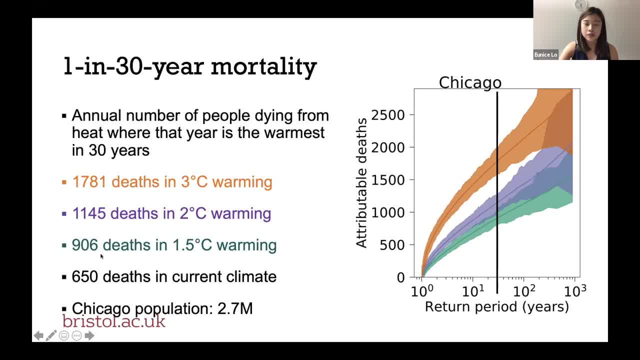 would be warmer already, And so we expect 906 deaths. These are all middle estimates And in a two-degree world, a lot more deaths- over 1,000 deaths- And in a three-degree world, even more: 1,781 heat-related deaths associated. 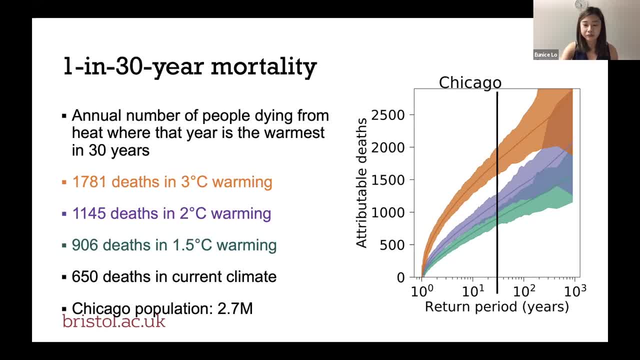 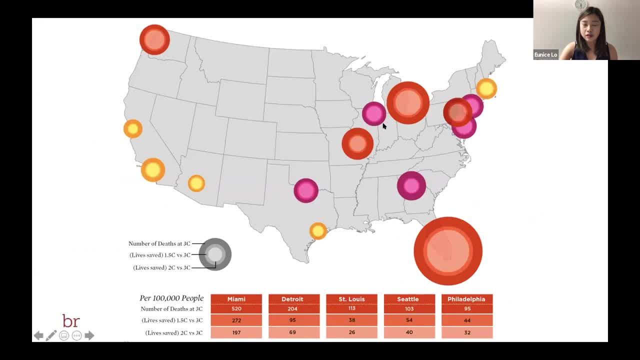 with a heat wave that comes back once every 30 years. So this is a case study for Chicago. We looked at all 15 cities in the United States And this is a summary figure. These are all number of deaths per 100,000 people. 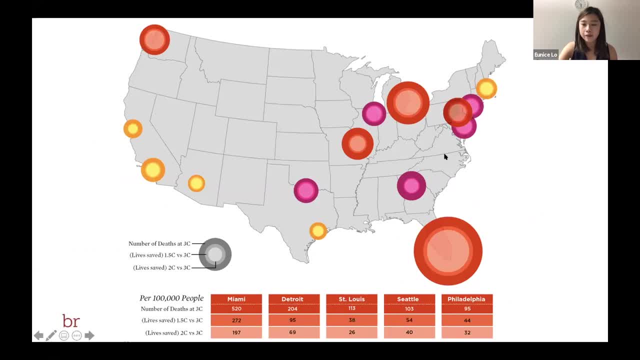 So they're normalized by the population of the cities. So each bubble, the outer circle on each city, indicates the number of deaths at three degrees warming. So the larger the circle, the more people per 100,000 people are expected to be adversely affected by three-degree. 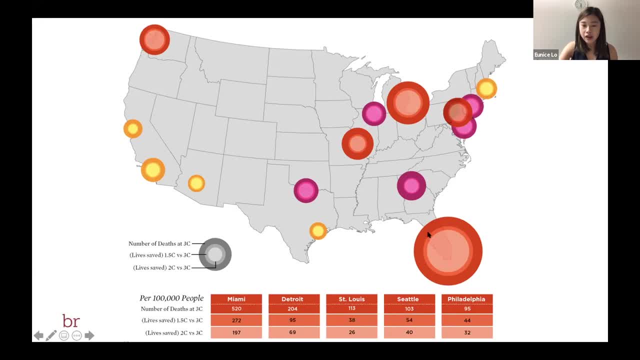 warming. The middle circle, the size of it, indicates how many lives could be saved by mitigating three degrees warming down to one and a half degrees, And the inner circle shows the number of lives that could be saved by mitigating three-degree warming. 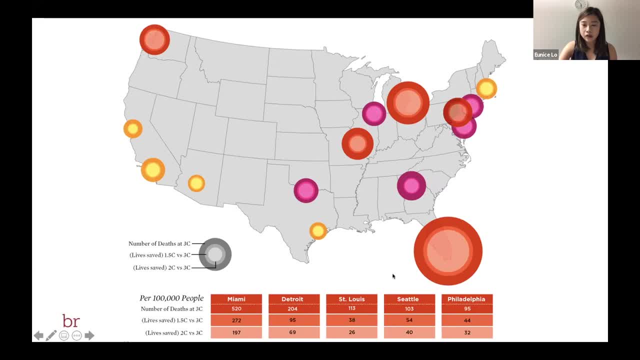 down to two degrees warming. So global warming- and also mitigation- has the largest impact on heat-related mortality in Miami And Detroit and so on. But for all of these cities we are expecting lives that could be saved in a one and a half degree. 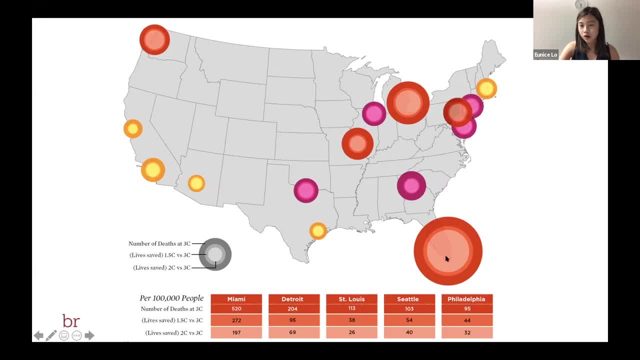 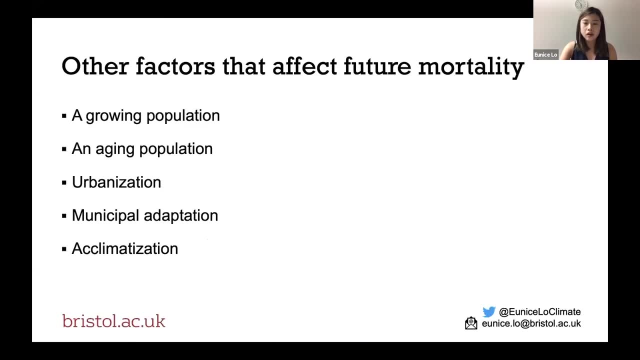 world and a two-degree world, And in a one and a half degree world we could be saving more lives in all of the cities compared to the other targets in the Paris Agreement. So there are other factors that could affect future mortality that I haven't looked at. 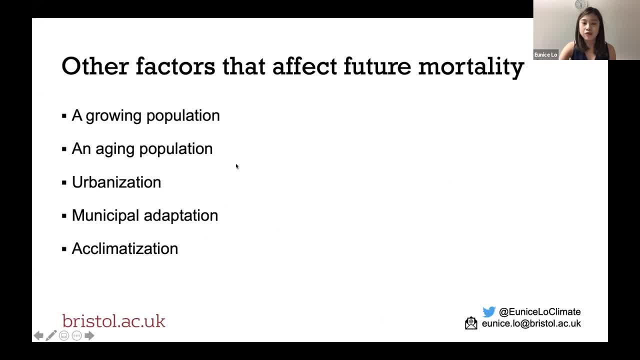 So this is the limitation of this study. Of course, if we have a growing population and aging population, we could have a more vulnerable population to heat or just high exposure. just because you have more people, Urbanization can increase urban temperatures compared to rural areas. 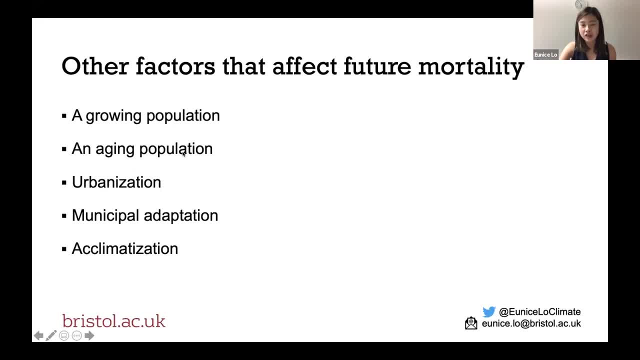 So that could exacerbate the impacts of heat waves and heat events. Adaptation, on the other hand, could reduce the impacts of extreme heat on health, and also people can actually, over time, start to get used to higher temperatures, And that's something that we didn't look at. 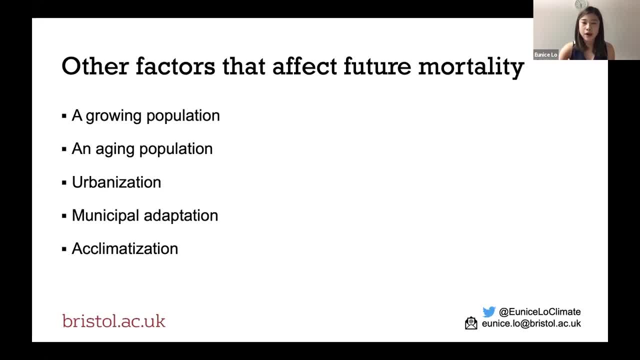 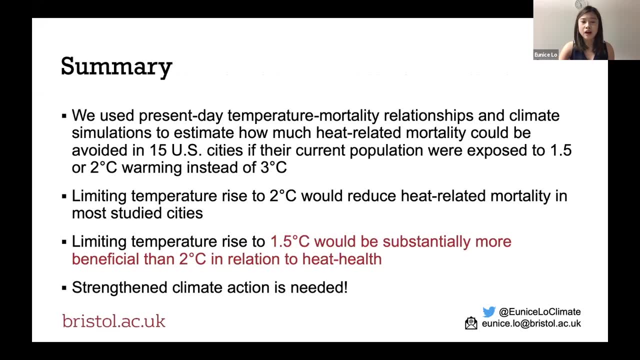 But we wanted to focus on solely the impacts of climate change- and also mitigation- on heat-related mortality. So this is the summary slide. Basically, we used present-day relationships between temperature mortality and also future climate simulations to estimate how much heat related mortality could be avoided in 15 cities. 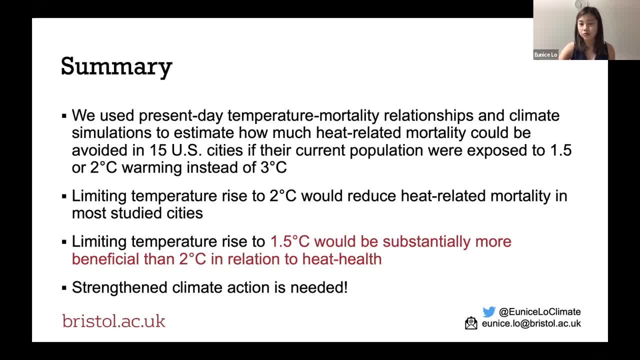 in the United States if their current populations were exposed to different warmings instead of 3 degrees, Limiting temperature rise to 2 degrees, which is one of the Paris Agreement's threshold, would reduce heat-related mortality, But limiting temperature rise to 1 and 1. 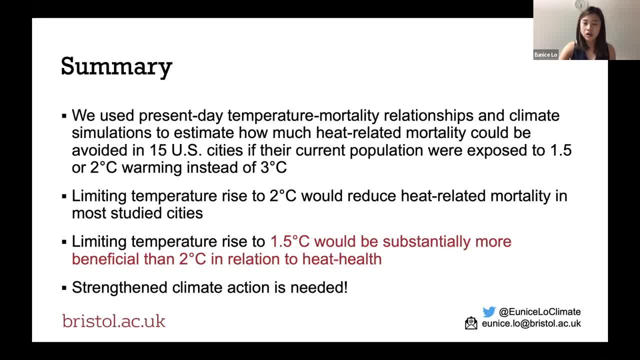 1⁄2 degrees, which is the more ambitious target, would be substantially more beneficial than 2 degrees in relation to heat health. So we do need to have strengthened climate action within the Paris Agreement or outside on all levels: on personal level, on the state level, national level. 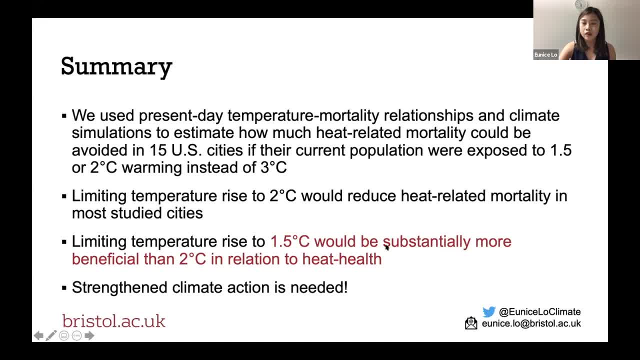 and also international level, in order to avoid the adverse impacts of extreme heat and global warming on human health. And that would be the end of my presentation, Thank you. Thank you so much, Dr Loh. Now it's time for our Q&A session. 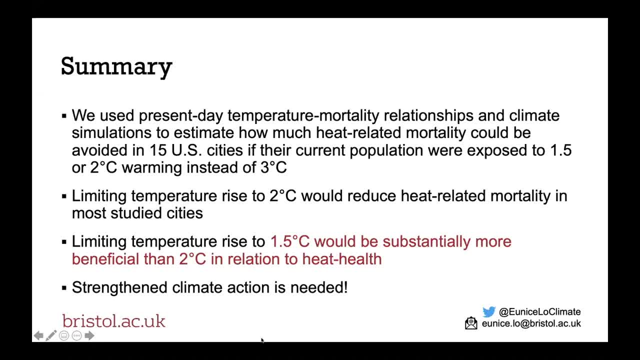 You may type your questions through the Q&A feature available on the menu bar at the top of your window. We will get to as many comments and questions as we can. Ted, would you like to start reading out one of the questions for us? 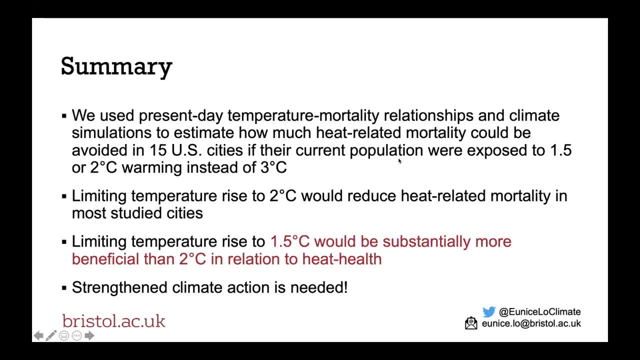 Yeah, sure, Thank you very much for your wonderful presentations And thanks for the people who have offered up some questions. Here's one that I think probably goes to Greg. It has to do with environmental justice impact and, in mapping, wondering whether you have you know. 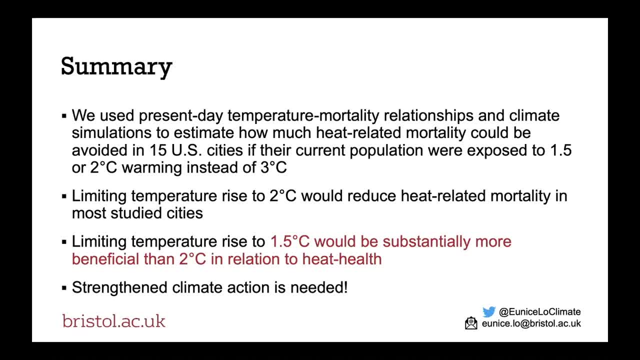 looked at population level socioeconomic status in study counties And I would add to that whether or not you were able to look at the impact of air pollution and how its impact on preterm birth, for example, might have affected your findings. I noticed that Rish did say that they had corrected. 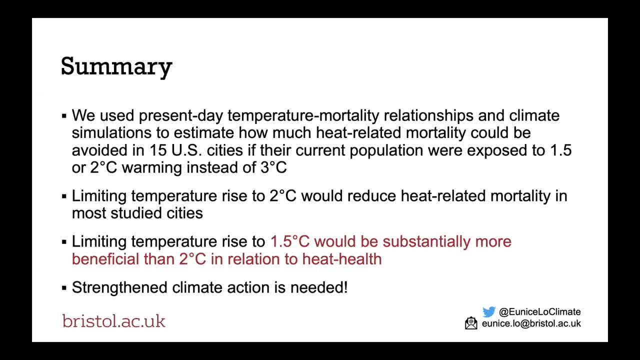 for air pollution, but I didn't see it in yours, Greg. OK, thanks, Ted, That's both correct, Both great questions. Let me take the air pollution one first, because that's the one I have an easy answer to. 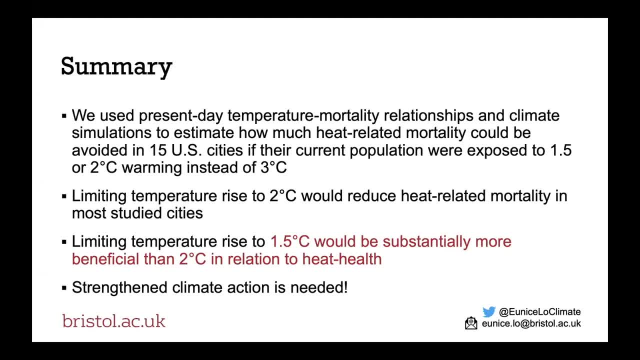 So we did adjust for potential confounding by air pollution, because the temperature and air pollution can be correlated And we did not see that the adjusted results or the results further adjusting for air pollution were not substantially different. So that reassured us that these are not due to air pollution. 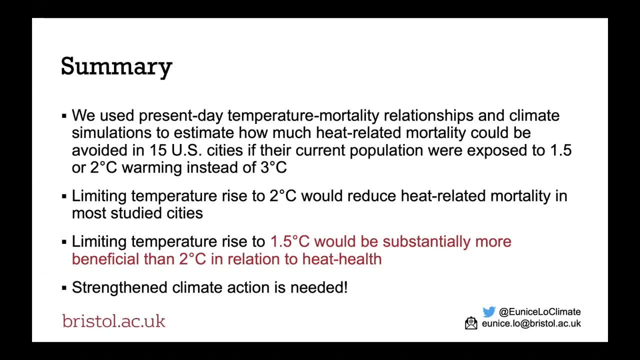 but we didn't look at the main effect of air pollution. There's, of course, a large literature showing that air pollution can be a risk factor both for preterm birth and lower birth weight. In terms of the socioeconomic piece, I think that's a great question. 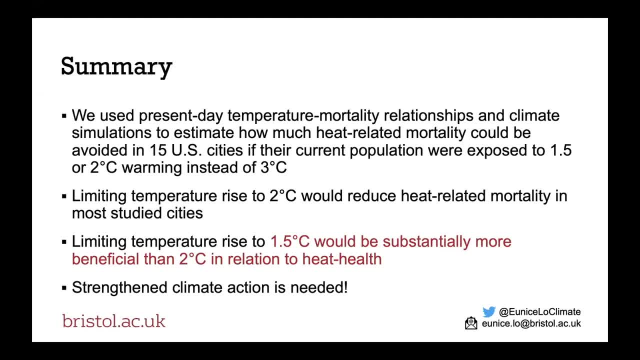 Our more recent work with a new postdoc in my group, Keith Spangler, has been looking, both in New England initially and now nationally, at how some of these temperature-related health effects vary, using the CDC's social vulnerability index as a marker that incorporates socioeconomic status. 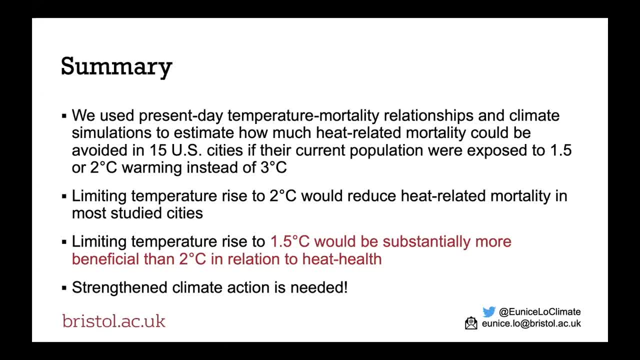 and additional factors. So I don't have an answer for that yet, but stay tuned, Thank you. Another question that came in said that one of the problems with lowering the heat alert warning level is that if it happens too often, people will ignore it. 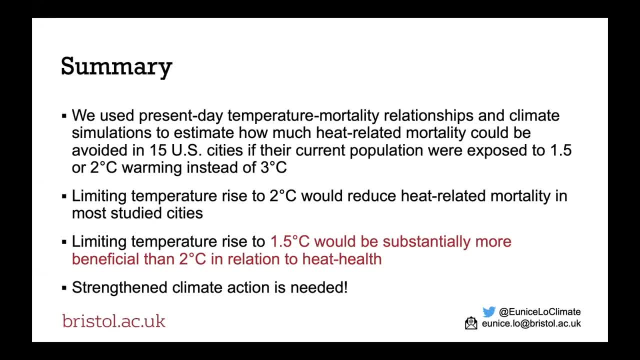 So, even though health effects can show up at a lower temperature, it may not be worth lowering the level. Do you have a comment on that, Rish? Oh, yes, I think that's a great question. That is definitely true, and that often comes up. 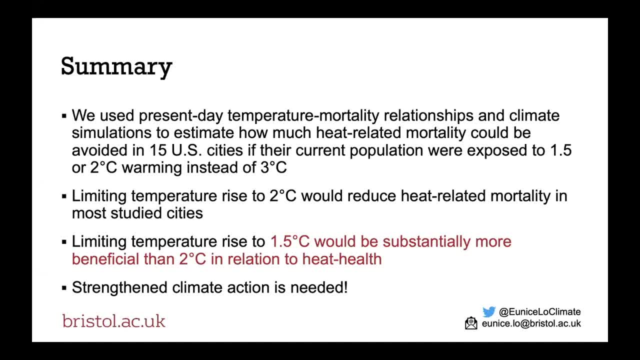 when we discuss this with our weather community and weather partners. So when you look at watch, warnings and advisories, so these are essentially at that particular temperature. the decision is a binary one. So whether you issue an alert, or issue an advisory or issue, 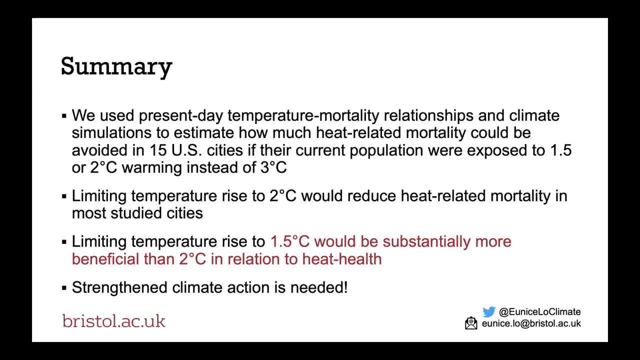 a warning. So, yes, from that standpoint, yeah, we don't want to lower that so that you have a lot more days as a heat alert days, But then what we're trying to do now was to look at a graduated alert framework, which 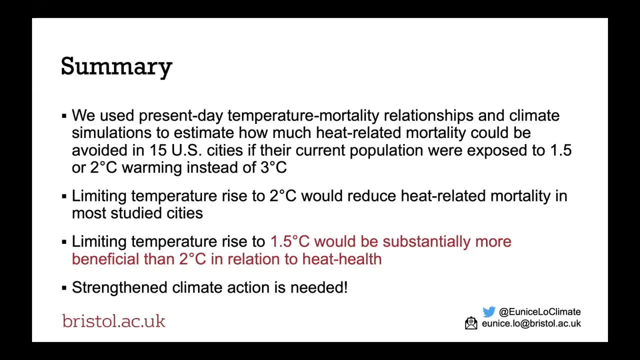 is similar to the AQI, where you have different color-coded ranges And also the interventions that we would propose for each of those ranges would be different and attuned to what the impact would be. So I think that's a great question. 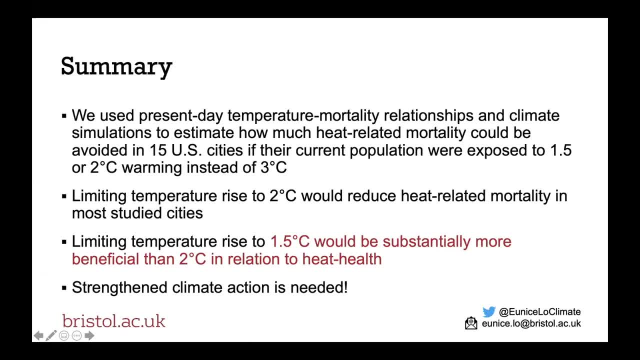 Thank you, And so, for those of you who are already on the panel, we're very happy to hear from you. It's very interesting to hear from you. We're very excited to be able to be here with you. We haven't been able to see you in a while. 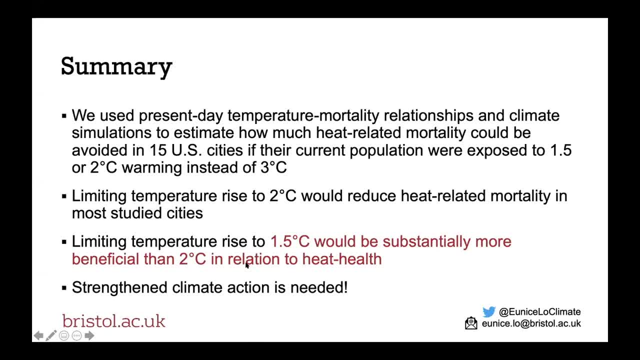 but at least we understand what impact would be at those scales. So that's sort of our way to address that is. obviously we understand warning fatigue is important, So it would be more to get the message across that there are wide varying public health interventions, so not everything. 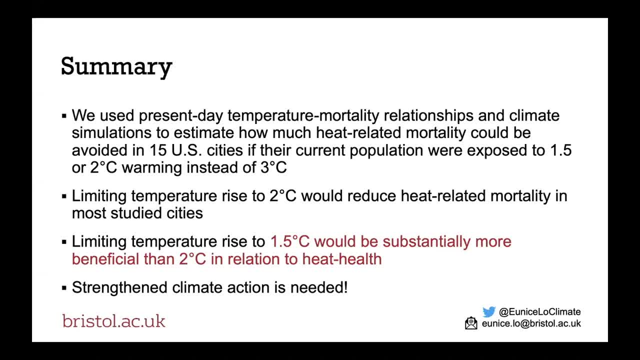 Thank you very much. Here's another question that came in. In cities, nighttime temperatures are increasing at a higher rate than daytime temperatures. Are there ways to parse out the data to better account for times of day where there are higher risks for certain vulnerable populations? 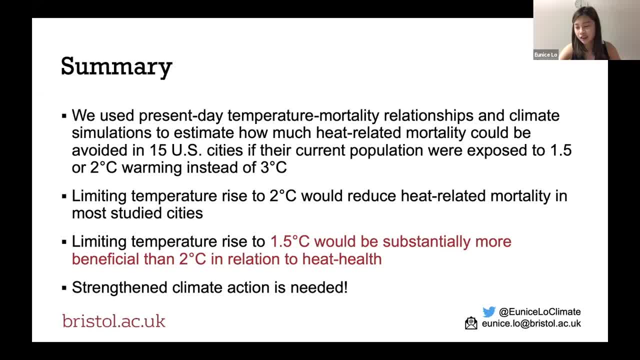 For whomever would like to tackle that. Yeah, I can take that. So yeah, if we have measurements of daytime and nighttime temperature, usually within the day, you have a measurement of maximum temperature of the day and minimum temperature of the day, then it is possible if you have data to look at the temperature mortality. 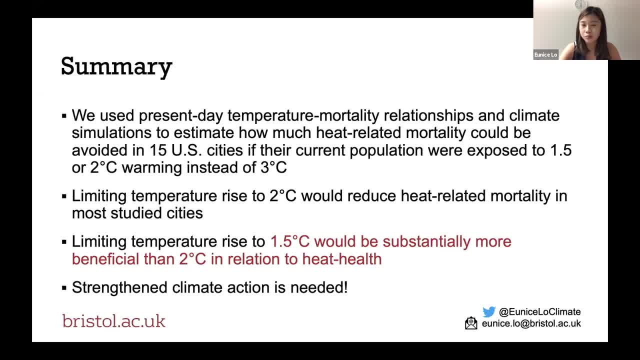 relationship or even other responses other than mortality in the exposure response relationship and to kind of parse out the different impacts of daytime and nighttime temperatures on health. Thank you, Here's a question for Greg. Did your group consider adjusting for air conditioning prevalence in different regions? 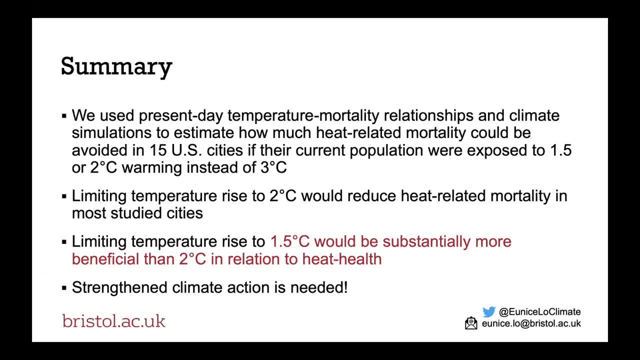 among different populations. Thanks, So it's a great idea. So there's two problems: One, that we don't have air conditioning. We don't know air conditioning prevalence with great resolution in terms of either space or time. So the American Community Survey or the American Housing Survey, I forget which one, does look. 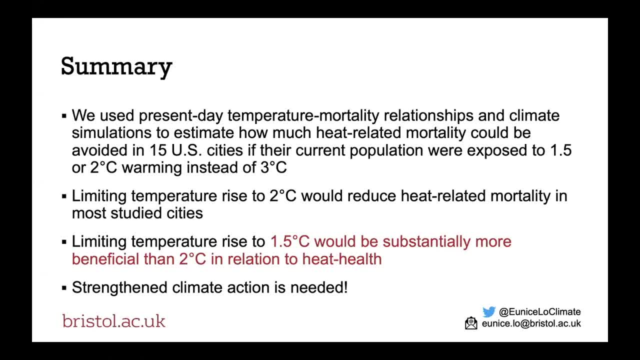 at air conditioning prevalence in selected cities in selected years. But there isn't a really great data set beyond that that would give us the resolution. And also, even within a county air conditioning prevalence is going to vary quite a bit and we don't know with this particular data set. we don't know that. 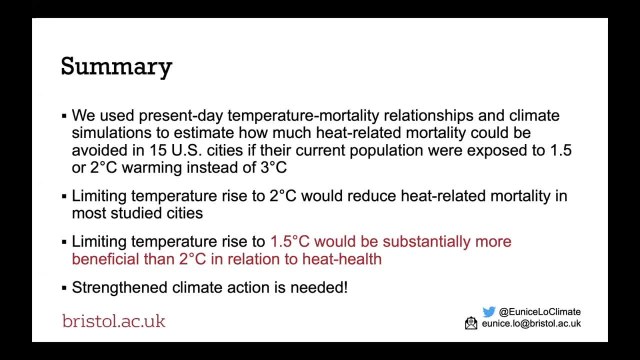 So I think it's a great question and a great point and I think it's something we want to figure out how to do better. I think there are studies from New York City where they've done survey work in selected cities in California also survey work where they have pretty detailed information across. 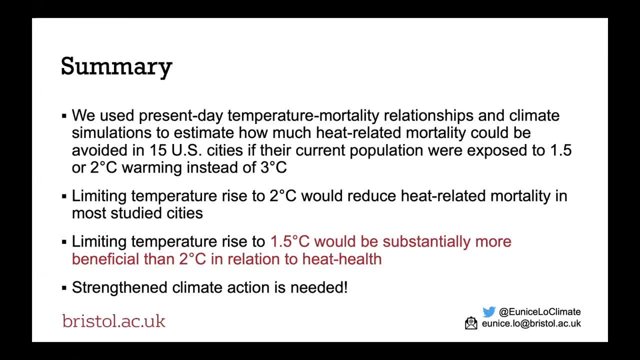 both space and time about air conditioning usage, And so we looked at those cities to guide our science on that, but there isn't a good national data set available for them. Thanks, Another interesting question came in. has to do with what measures of morbidity might we? 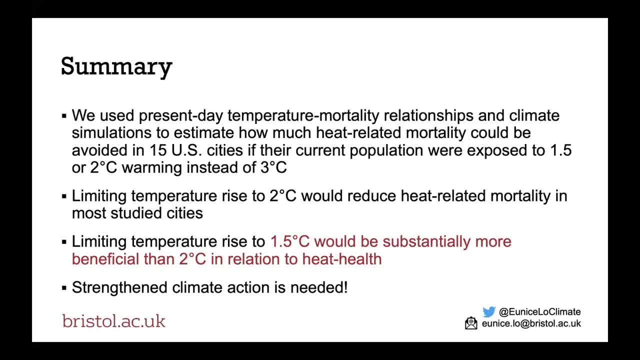 be looking at, And one suggestion is: might we consider taking a closer look at increasing rates of health and learning challenges among children as a function of testing? So we're looking at the temperature. I remember seeing a very recent news article about children in schools. 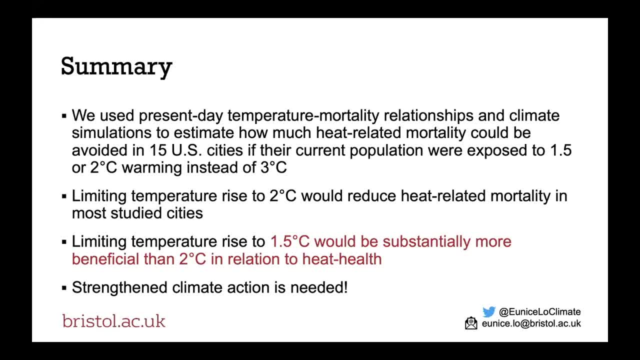 Yeah, so I guess I could comment on that. So right, I think there's a big problem. I think there's a big problem, a great deal of interest in studying the health effects of of extreme temperatures on kids, and there's very little data and i think that's a an area of interest. perhaps for you know some of the 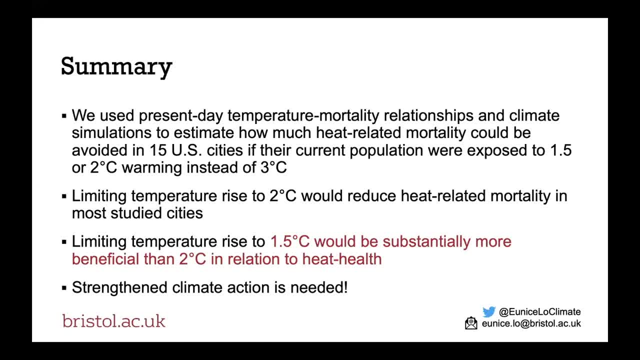 you know my colleagues on the presenter side and i'm sure for many of the audience members, i think it's an active area of research. we just haven't seen a lot of data on on what are, are the, the health effects? and as that emerges, then the question is when you think about heat warnings? 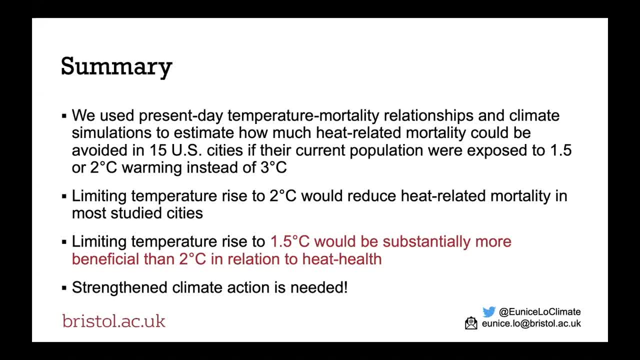 right now heat warnings are given um to an entire population and uh, there's sort of the the general population warnings and then for occupy in some occupational settings there's a different set of criteria and mechanisms for protecting those populations. but really, as we go forward it in 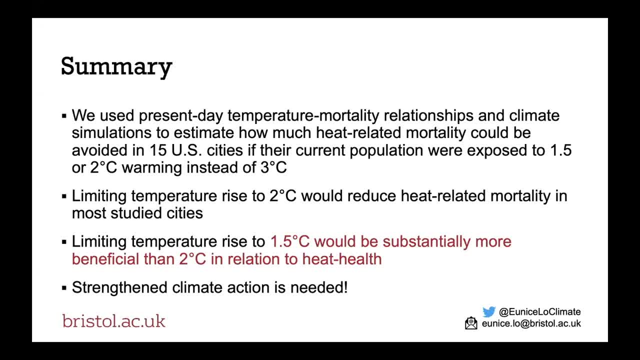 my mind, it would make sense to think of: uh, okay, that these are the conditions that are particularly dangerous for kids, uh, in many of which attend schools that are not air conditioned, uh, and where, whereas maybe other segments of the population aren't equally sensitive, or that the precautionary 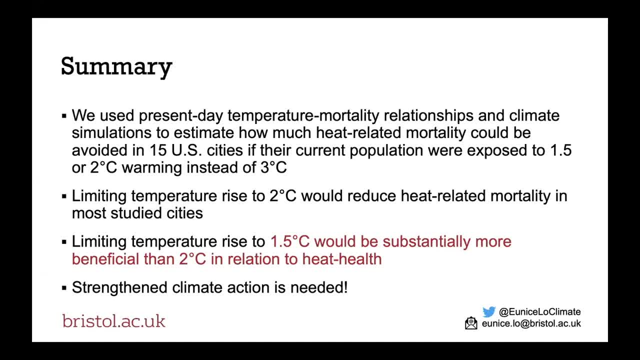 messaging and the actions taken might be different when you're thinking about kids versus elderly, versus outdoor workers versus pregnant women. So I think, over time, what we're going to see is a targeting, a specificity of the heat, of our efforts to mitigate the health impacts of heat. 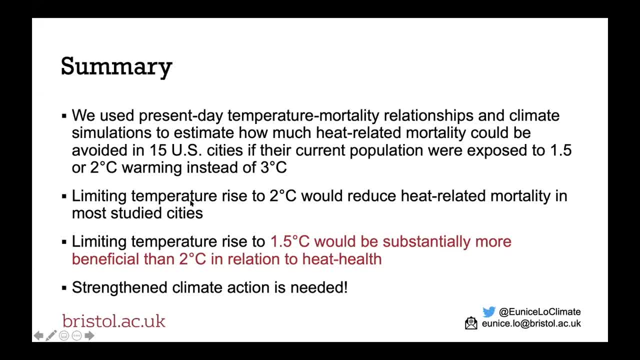 Thank you very much for that, And I think that brings us to the end of our time. I just want to thank all three presenters for wonderful presentations and very thought-provoking data presentation- And I'm going to turn it back to you, Hannah. 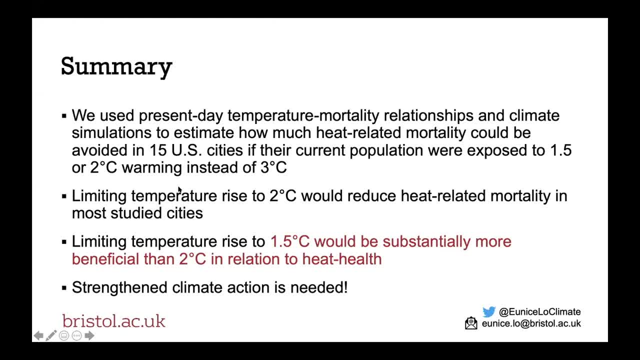 Great. Thank you so much, Ted. We're approaching the end of today's webinar. A video recording will be available on SHEA's website And tomorrow you'll receive an email containing the link to the video. SHEA's next webinar will take place September 24th and is titled Disrupting Cancer: Systemic.